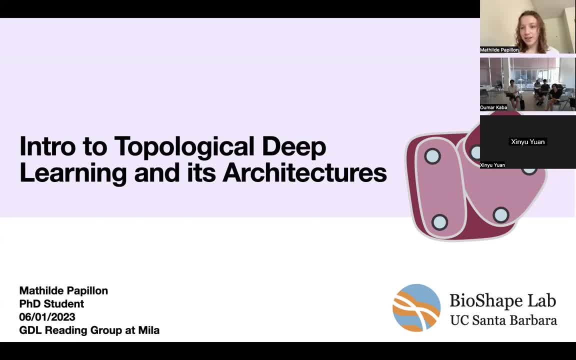 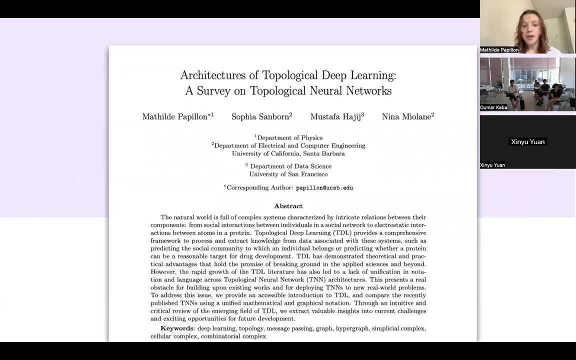 and the literature behind it. This work has come out of a literature review that we recently put out on our website. It's called Topological Deep Learning and the Literature Behind It. I think people are really excited about this field and see a lot of potential in this field. 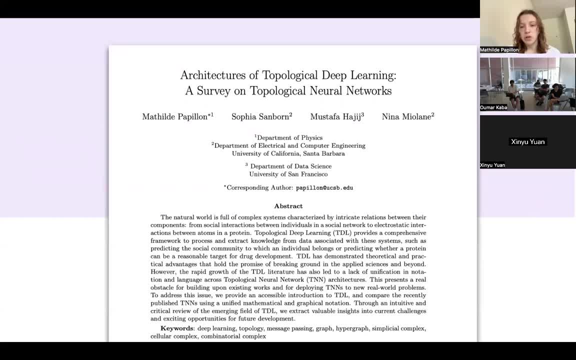 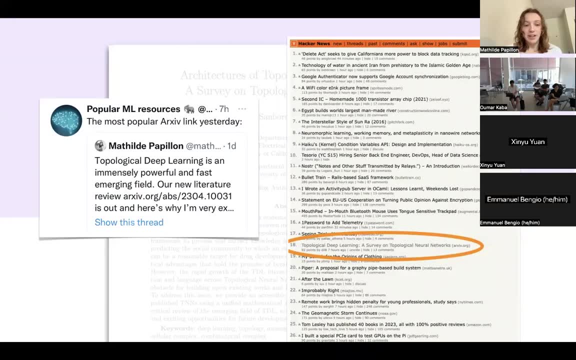 and it was really exciting to see so many people want to get involved The day that it came out. it was the most popular archive link on AI Twitter, which was crazy, and it made Hacker News, which was also really exciting, So hopefully I will. 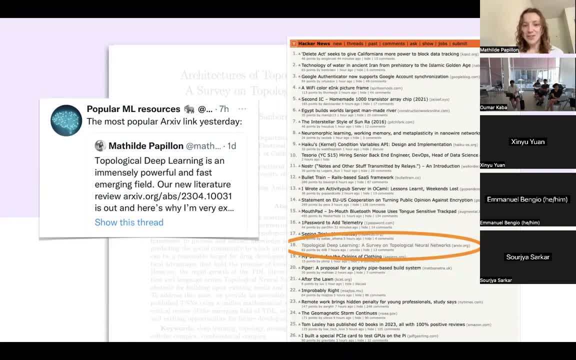 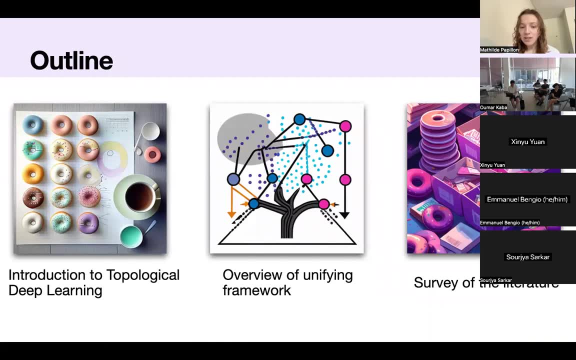 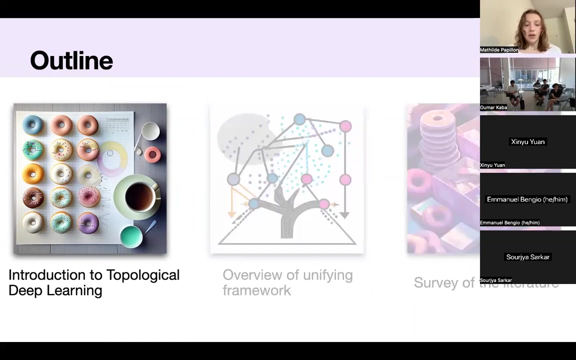 summarize the results of this literature review concisely. over the next hour I will go through an introduction and then build up a framework that we can use to systematically break down any topological neural network in the literature, and then we'll look at what the literature looks like to this current day. Okay, So to start explaining topological deep. 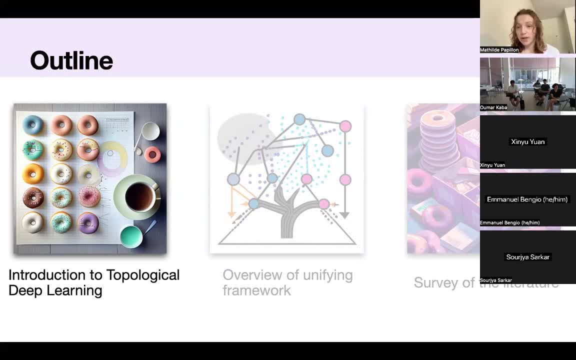 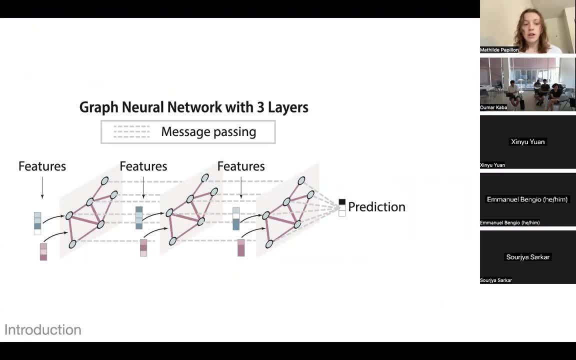 learning. I'm going to go ahead and start with the topological deep learning. I'm going to start with something that we might be familiar with called a graph neural network. So, as you might know, in a graph neural network, a graph supports our input data. 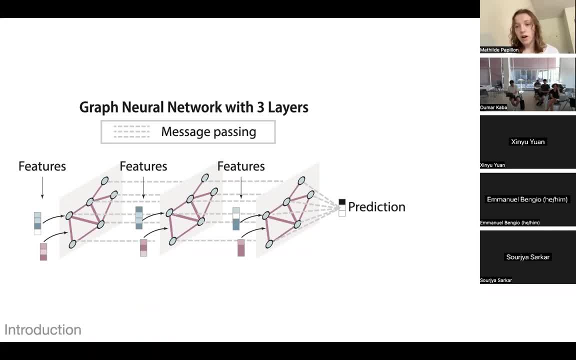 So all of our input data is represented on features on either nodes or edges of the graph, And at each layer of the graph you are updating those features by, you can imagine, passing messages between the nodes, And this is maybe a little bit abstract. So let's draw a visualization of this. 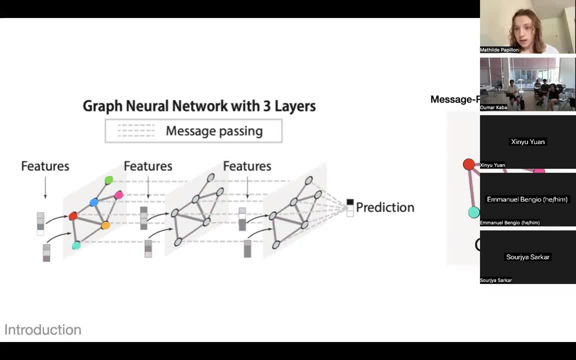 message passing scheme. So let's say that your input features on your nodes are some colors and each color represents whatever- some scalar. This is your first layer. When you pass messages, you're going to send information through the edges of the graph, in this case, and update the color on each node. 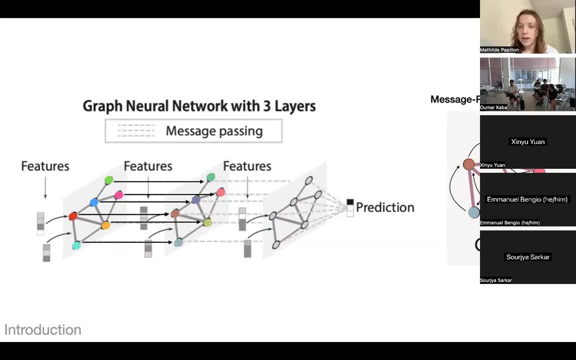 And that becomes what your graph looks like at your second layer. And then you keep going with this process through multiple layers until you hit the last layer where information is aggregated across the graph into a single prediction. So that's the graph. neural network- Graph. neural networks have been very powerful and very popular. 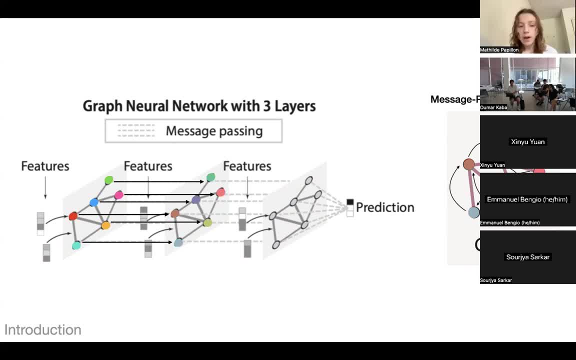 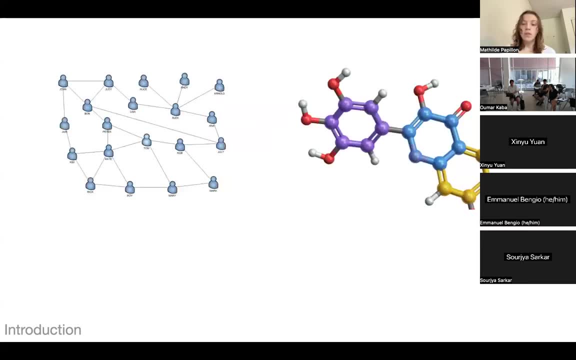 in deep learning in the last years. However, they might not be the best choice for certain data sets, And let me give you some examples. So what if you have a social network of individuals connected by relationships on some social media platform, for example? or a molecule with atoms? 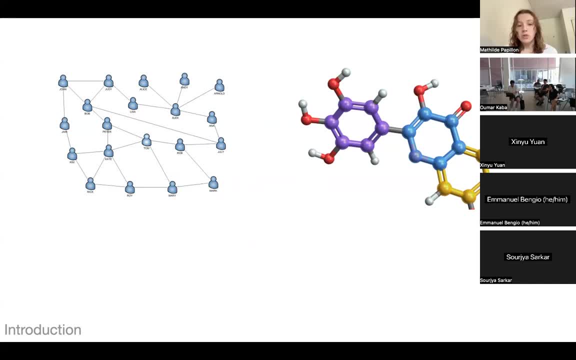 connected by bonds. In both of these situations, pairwise relationships are very important to describing your graph, But also you have relationships that go beyond pairwise connections. What if you have a group of four individuals that all share something in common, that are part of the same group? on social media, for example, A graph can't represent that. 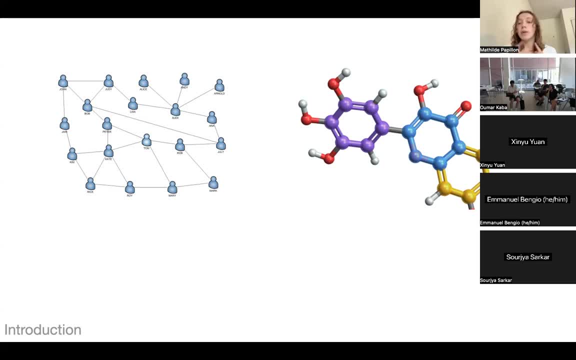 type of information easily. You can only have pairwise connections, So telling your graph- all of these four people share something in common- is quite difficult. Similarly, in a molecule, a benzene ring is a very important piece of information to what your molecule can do. right, Whether or not your molecule has a benzene ring. 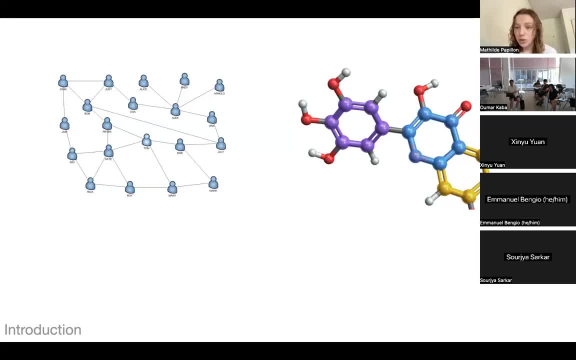 inherently changes its functionality. However, in a graph, you have no way of encoding that information directly, unless you tweak your graph a little bit or change your input data. So instead, what if we had a domain beyond a graph that could encode these higher-order? 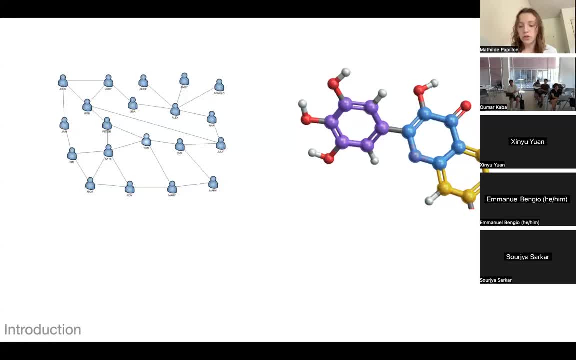 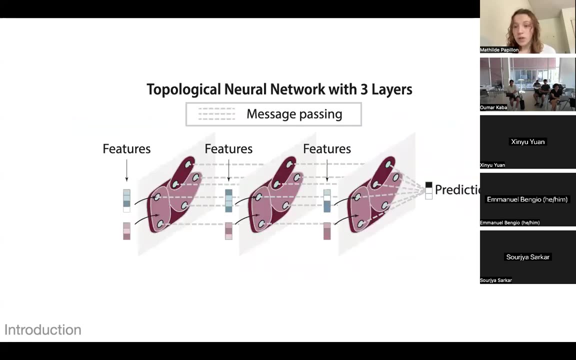 relationships like benzenes or groups of people in a social network, And that's what a topological neural network is. So a TNN generalizes a graph neural network by representing higher-order relations. So this is what a topological neural network can look like. 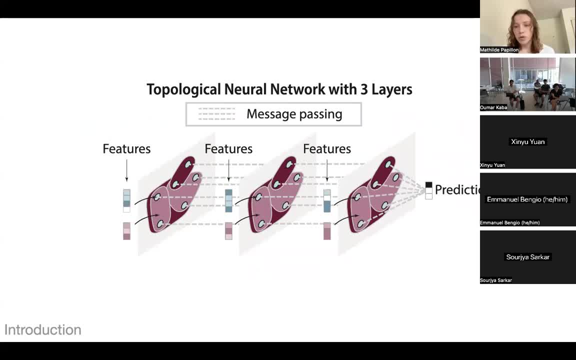 In this situation, we have the same sort of message passing, happening at every single layer, except now, instead of being constrained to pairwise relationships between our nodes, you can have a relationship that connects three nodes at a time. You can have a relationship that is higher rank than another relationship, and we'll get into what. 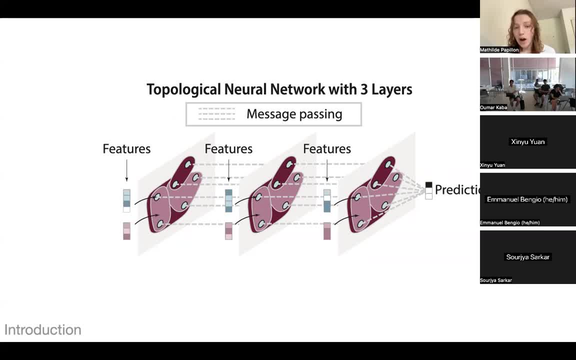 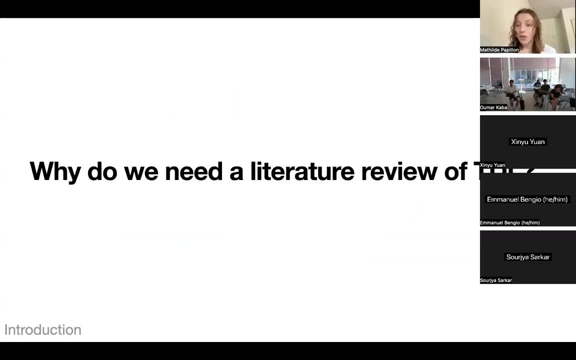 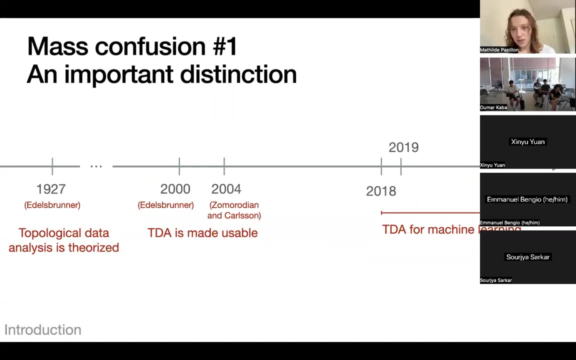 all of that means. But off the bat, I hope you can see how a topological neural network can be more powerful and more expressive than a graphical network. Okay, so now, why a literature review of topological deep learning? There are two big reasons for this. They're both sort of mass confusions that have hindered 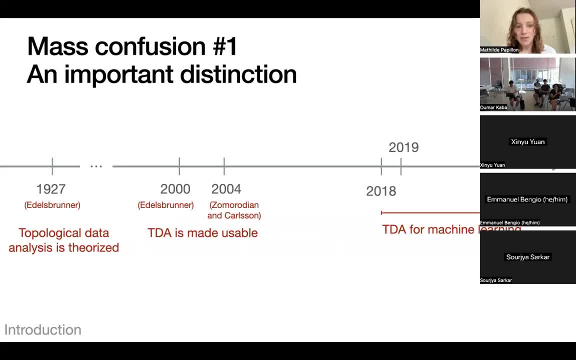 the accessibility of the field. The first mass confusion is the distinction with topological data analysis or TDA. Maybe you've heard of TDA before. it's been around for about a century and has been applied in machine learning for about the 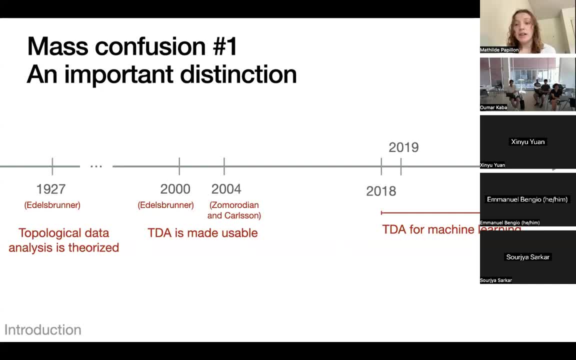 last five years. TDA is inherently a data processing method that has nothing to do with machine learning. So what people do is, for example, pre-process their data using TDA or will use TDA to help select a specific model during training, But the model they're 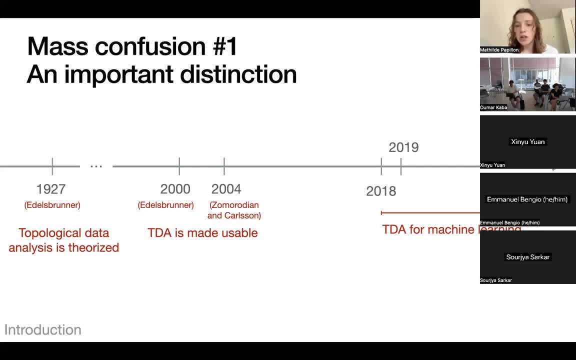 using inherently. the machine learning model that is being used remains mostly standard or classical. In parallel to the TDA field, deep learning on topological spaces or topological neural networks have started emerging in the last four years or so, And both of these fields 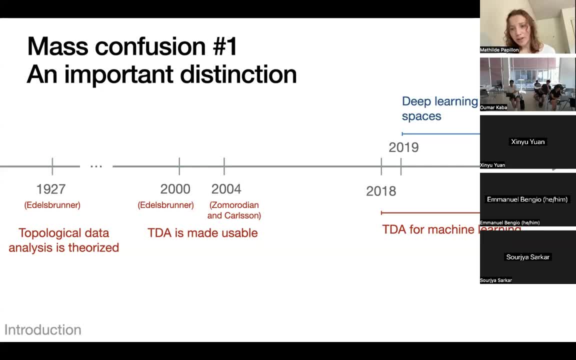 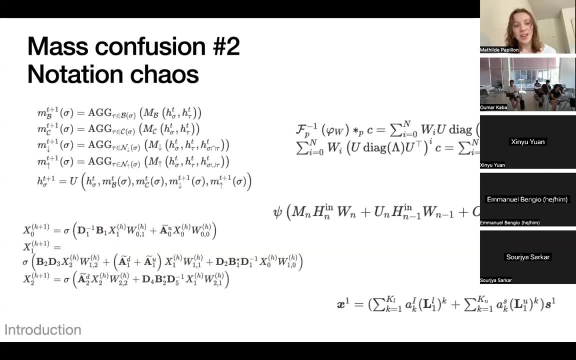 are topological machine learning to some extent, but it can be quite confusing to distinguish which is which. Hence the need for literature review of the blue field. The second mass confusion is notation chaos. The field's mathematical inclination has made it so that a lot of papers come up with their own notation that is best suited to their own. 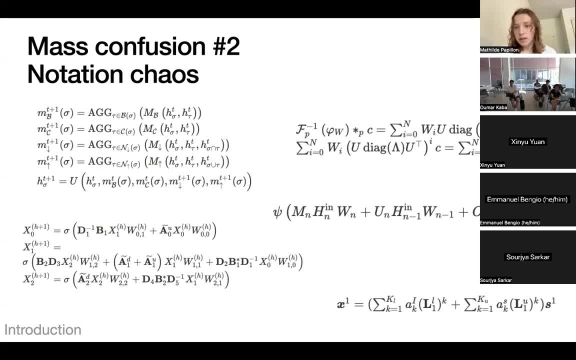 application. But what this means is that when you start reading the literature, every single paper uses a slightly different notation. And that means that when you start reading the literature, every single paper uses a slightly different notation. All the notations on this slide. 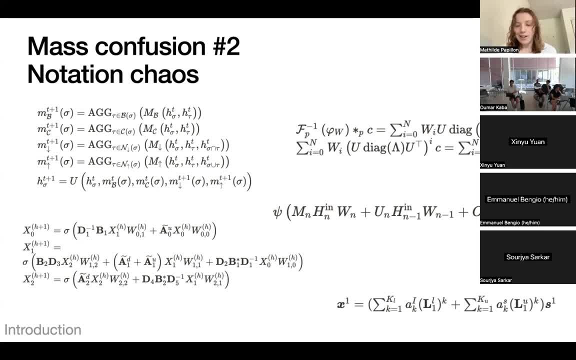 represent the same thing and nothing looks the same. So for a practitioner interested in using topological neural networks, this makes it really difficult to navigate the field. So through literature review we hope to unify the field and make it very clear which questions 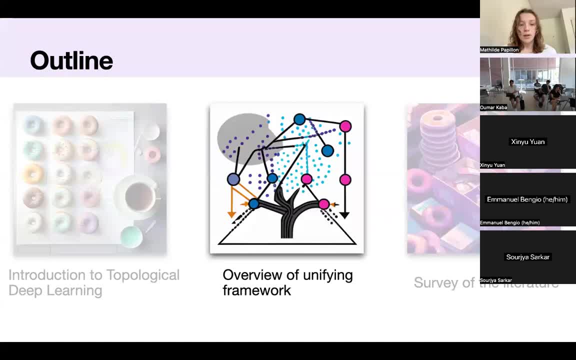 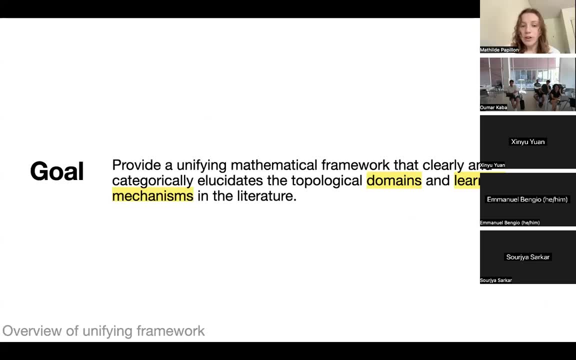 have been answered and which questions have not been answered. Okay, so on to the unifying framework. The goal of our framework is to clearly and categorically elucidate the topological domains and learning mechanisms in the literature. We're going to break this framework down into three. 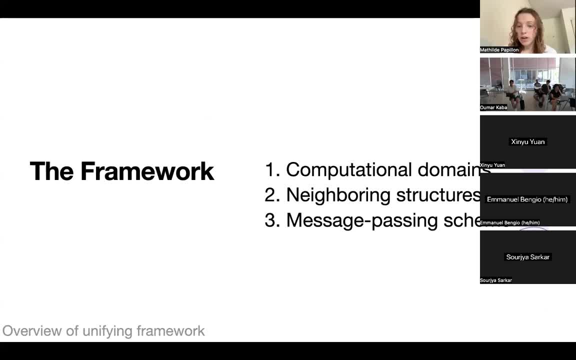 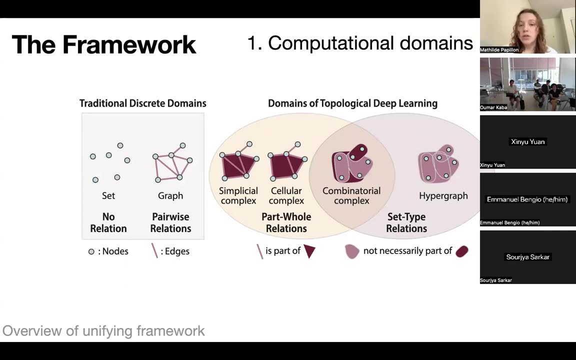 parts: The domain of our neural network, its neighboring structures and the message passing scheme. Let's start with domains, So I hinted at this earlier. A graph is a domain, but it is a traditional discrete domain. It only allows for pairwise relations and it only allows 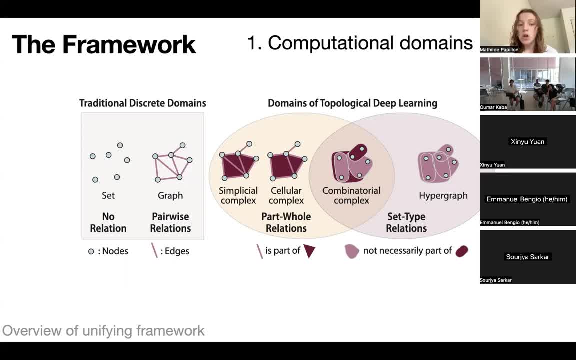 for edges. In topological deep learning we generalize this domain using more flexible, higher-order relations, And in particular there are two kind of relations that we can use to do this. Part-whole relations allow us to add extra surfaces and volumes that are sort of geometrically constrained by edges. So, for example, 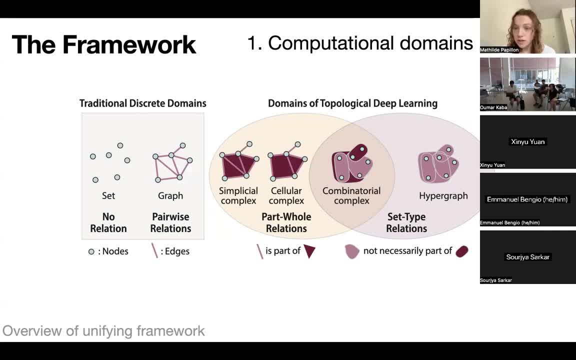 in a simplicial complex, you can add triangles that are bounded by three edges, And now your triangle is a feature of your topological neural network, just like the node is and just like the edge is In a cellular complex. you have a little bit more flexibility in the sense that you don't 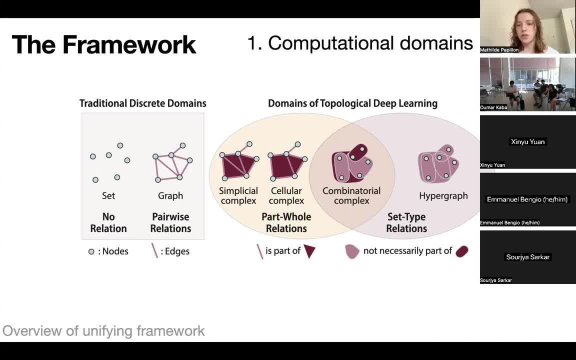 need to have triangles, only You can have triangles. but you don't need to have triangles, only You can have squares or any other shape. And you can imagine, if we went in three dimensions you could have cubes, for example, inside of your complex, inside of your domain. The other relation: 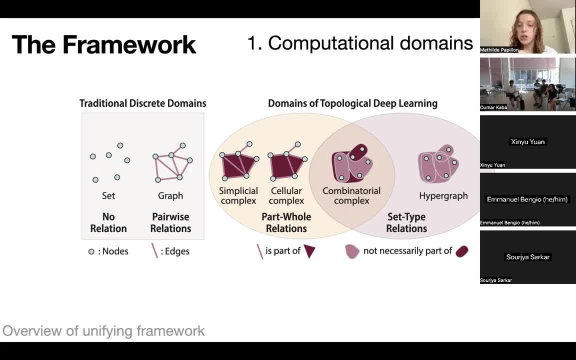 is called a set-type relation. In a set-type relation, you can have any amount of nodes in one edge, So it's super flexible. The hypergraph that we have here, for example, has three nodes in an edge, four nodes in an edge. There are no constraints, However, you'll notice. 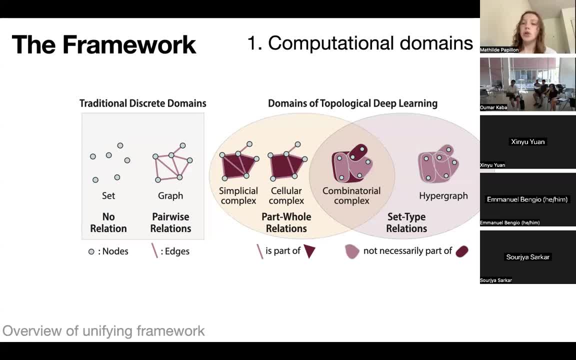 that in a hypergraph we're still constrained to nodes and edges. We don't have access to surfaces, faces or volumes. A combinatorial complex is kind of the holy grail, because it combines both part-whole relations and set-type relations. So now we have all the flexibility. 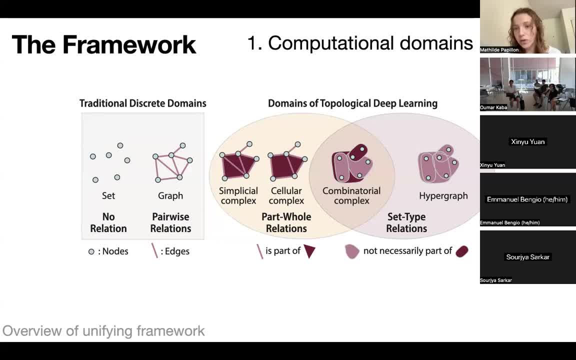 of a hypergraph in the sense that any node has three nodes in an edge. So now we have all the flexibility of a hypergraph in the sense that any node has three nodes in an edge. So now we have node can be connected to any node and we also have this idea of rank, this idea of 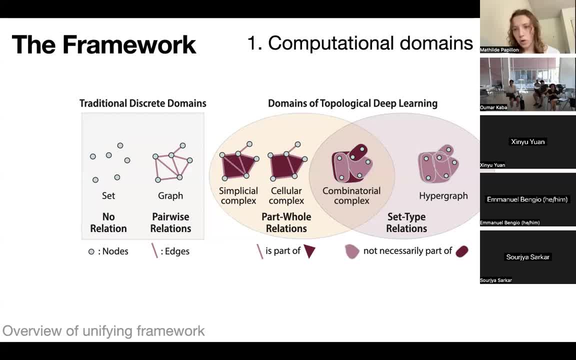 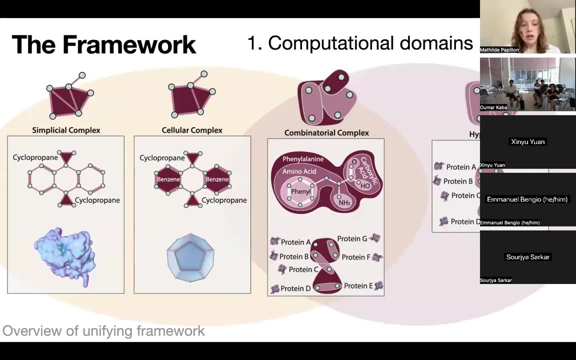 edges, surfaces and volumes from part-whole relations. So this might sound a little bit abstract so far, so let's look at what these domains look like for real datasets. Okay so, starting with part-whole relations, simplicial and cellular complexes are really. 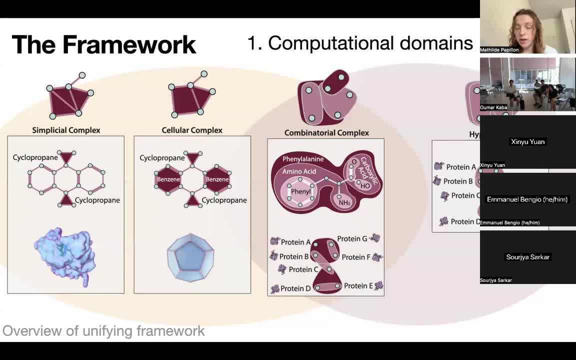 powerful for datasets that have geometric structure. For example, if you have a molecule, you can represent the physical connections of your molecule as well as the physical surfaces, like a benzene ring, for example, or cyclopropane of your molecule inside of your complex. 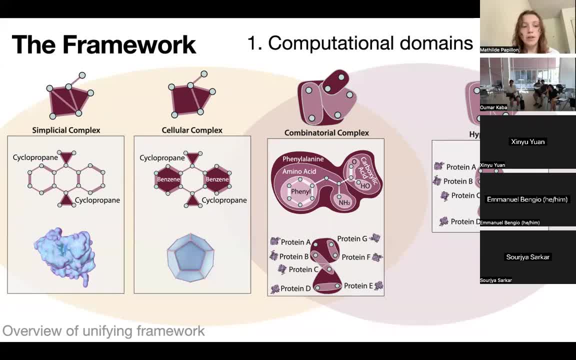 These are also really powerful for meshes. so bottom left there is a mesh of a protein surface And it's a simplicial complex because every single face of the mesh is a triangle. In the cellular complex case you could have a mesh with pentagons or octagons and be much. 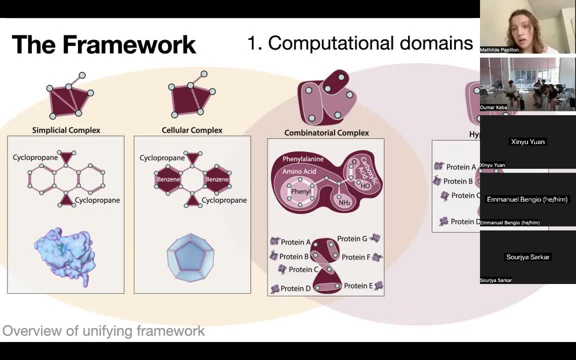 more flexible. In the hypergraph case we have an example of a protein network where you can have multiple proteins interacting through a hyperedge with multiple proteins. So maybe in a protein network you want to encode the fact that proteins A, B, C and 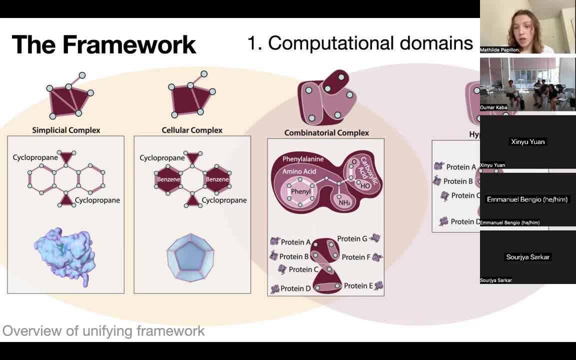 D are inherently connected in some way, but that doesn't necessarily imply that A and B are connected. B and C are connected and C and D are connected. So you can skip the pairwise relations and just encode groups as singular relations. And then finally the combinatorial complex. What we want to do is look at the homogenous connection between the two and see what happens, So we can look at the homogenous connection between the two. So we can look at the homogenous connection between the two, And then we can look at the homogenous connection between the two. 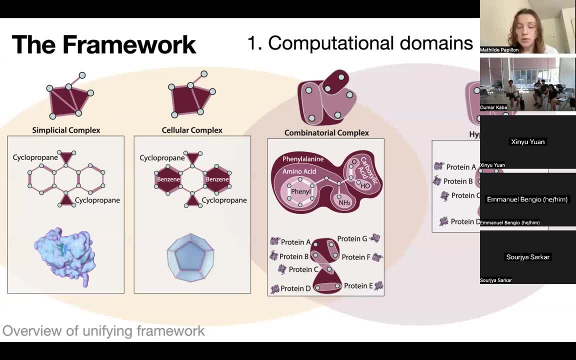 complex is the most important domain in the sense that it's the most general, And here we have access to both the geometric relations. So, for example, our molecule has geometric bonds that we're encoding And we have access to the functional relations where we can encode the 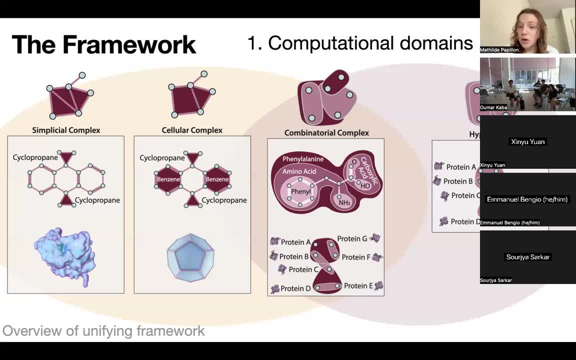 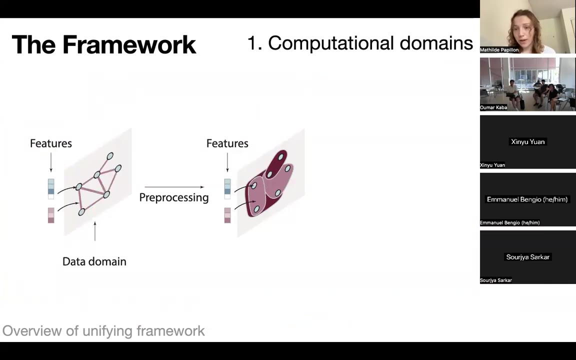 fact that a certain group of atoms is an amino acid or a certain group of atoms is a carboxylic acid, And this can be really powerful to encode both the physical nature of your molecule but also the functional nature of it. Okay, so now we have our domains And say we've picked our domain. 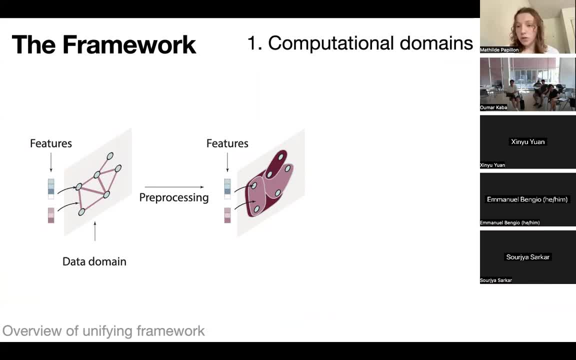 for our data set. We say: the combinatorial complex is what I need to encode all the important information on my data set. So the first step is to lift our domain. A lot of data sets you get will be only in graph format, for example. So during preprocessing, 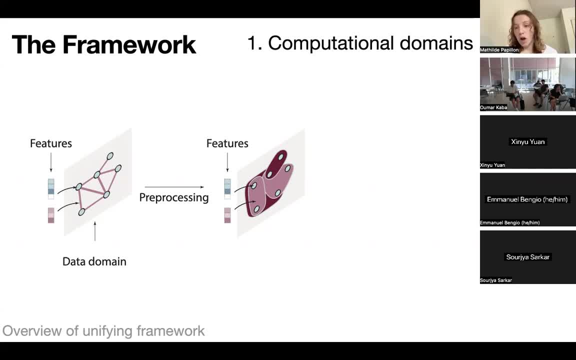 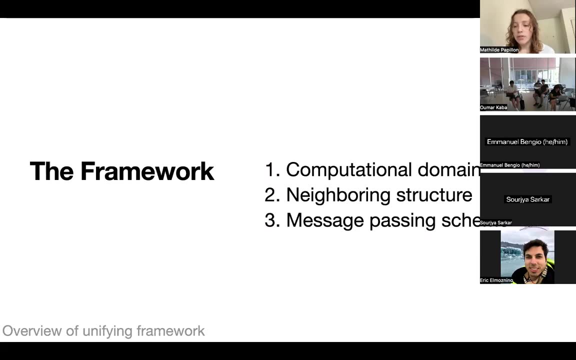 we will lift it into our combinatorial complex domain And at that point we feed it through a topological neural network. Okay, so that was our domains. The next thing we have to figure out is how information travels over the domain, And this is encoded in our neighboring structures. 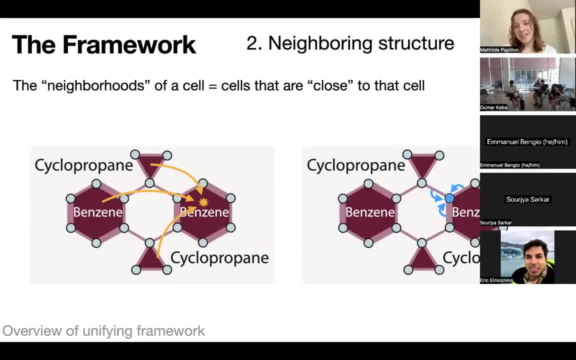 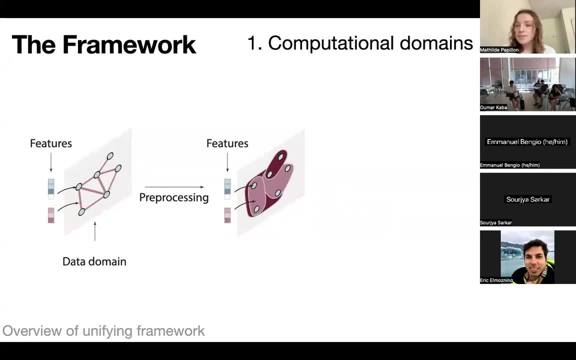 Now, if I may, I have a question about this lifting procedure. So how is that done? I feel like maybe there's not a unique way to do it or there are subtleties. Absolutely Yeah, there is no unique way to do it. There's a lot of research actually. 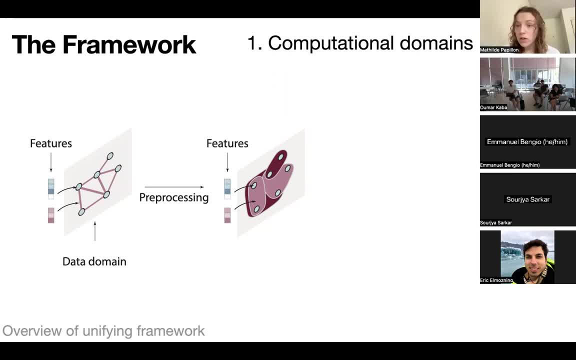 as to what the best way to do it is. You have to be careful because, for example, in the process of lifting into a graph, into a simplicial complex, you don't want to be adding artificial relations in the sense that you could have a paper right that's written by three. 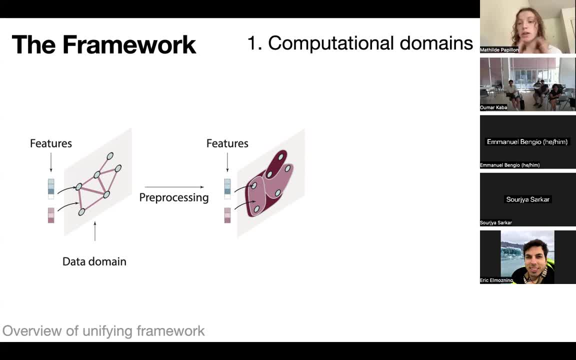 authors in a citation network. So in a citation network this will look like three authors that have one paper in common. So you'll see three edges In a simplicial complex that one paper becomes the surface connecting those three authors. However, you don't want to still have an artificial relationship. 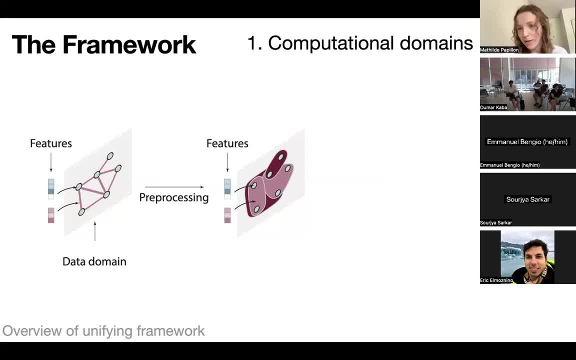 between authors A and B that have never written a paper together. But sometimes in the process of lifting into a simplicial complex, if you're not careful you can introduce these artificial features that didn't exist in the first place. So you definitely have to be careful. I think this is mostly these lifting operations have. 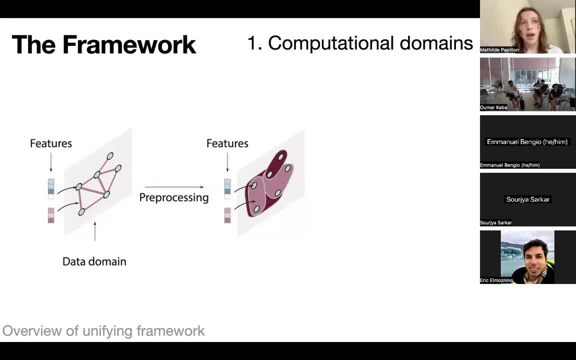 mostly been done with citation networks so far and some protein networks. A lot of people don't even use the higher order features. They don't even use, like the surfaces or the faces or the volumes as input features, but rather they use them to. 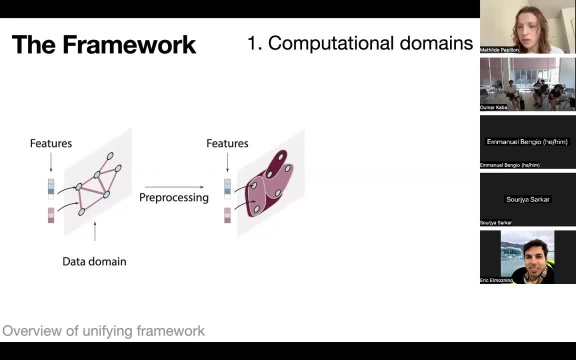 to be able to send messages with more flexibility on their domain. So you'll have a graph that is lifted into a higher order domain, but the edges or the faces or the volumes of that graph remain empty at input and are only used for computational purposes, if that makes sense. So there's a lot. 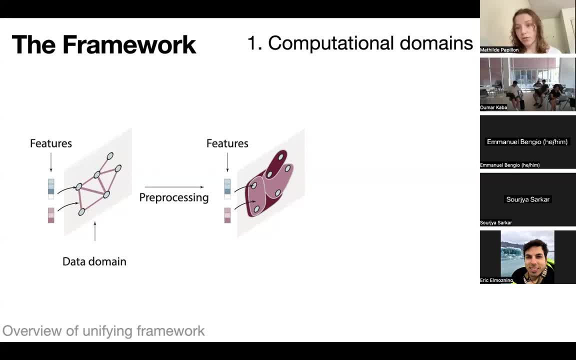 of different things that you can do and you're absolutely right. You have to be careful as to how you do it. I see, I see Makes sense. I see there's a question or comment by Emmanuel in the chat, If you want. 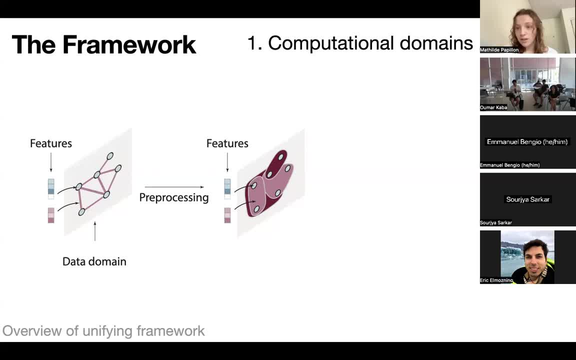 you can unmute and ask it directly, whatever you prefer. I can just read it, So let's see. So Emmanuel is saying I'm guessing there's an exponential explosion of possible relationship. How does lifting look like in terms of computational complexity? 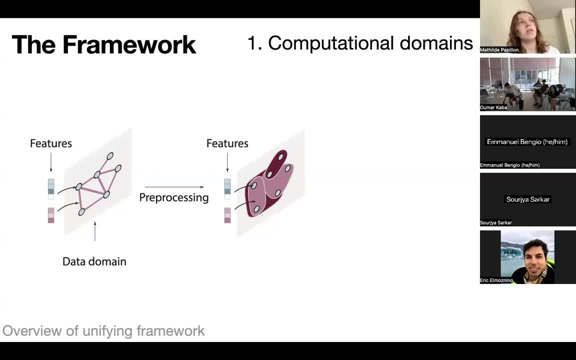 That's a good question. Lifting in terms of computational complexity really depends on how you're lifting, And there's a lot of different ways that you can do it, But in general, if you're working with a data set that already has its 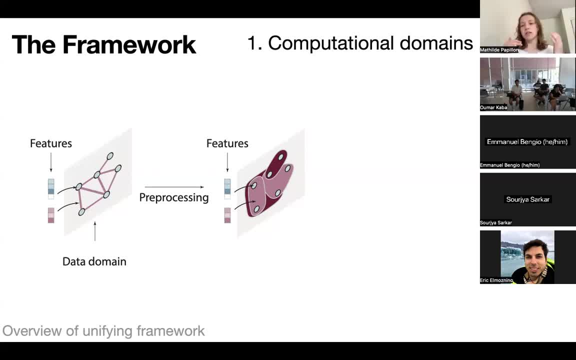 shared relationships encoded. so, for example, to come back to the citation network, if your nodes you already see which authors, group of authors, share a paper in common, then you don't need to go through all the possible nodes of the graph to know which ones are connected to which ones. 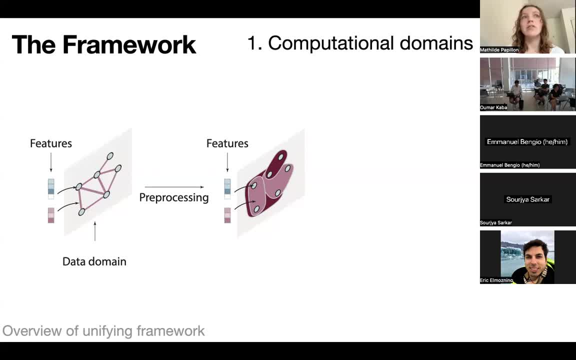 if that makes sense, So kind of similar to a multimodal graph where you have types of data associated to each node. So if you're working with a data set that already has its shared relationships, you can have a topological domain that is, aggregating information across nodes. that 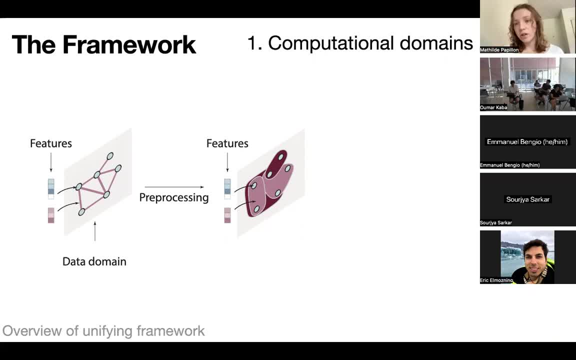 already share similar types of information. What I've seen so far in terms of working with data sets is that the most complicated part is that the biggest hurdle is not the computational complexity, but it's the decisions you have to make in terms of which faces or surfaces should be given features and which should not, For example, in a mesh. 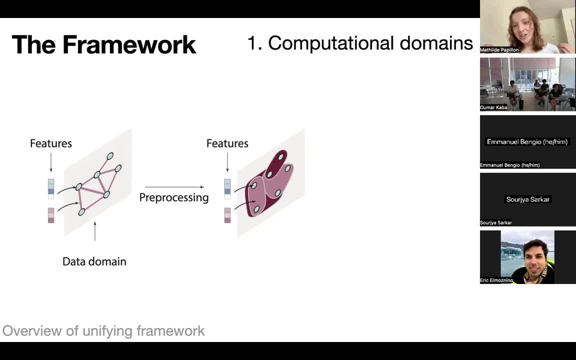 do you put features on all of the triangles of your mesh or only on certain triangles, for example? And that's just sort of a decision the practitioner has to make. Does that make sense? I see your question. I think it's a great answer. So, yeah, thank you, You can go ahead. 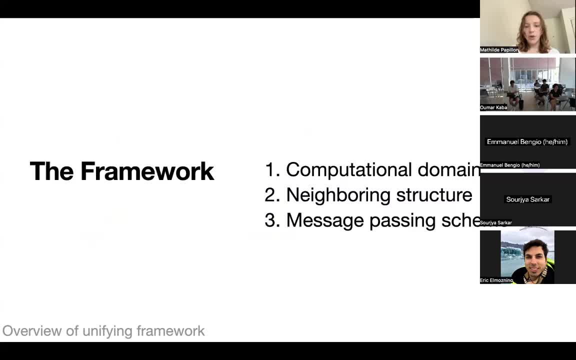 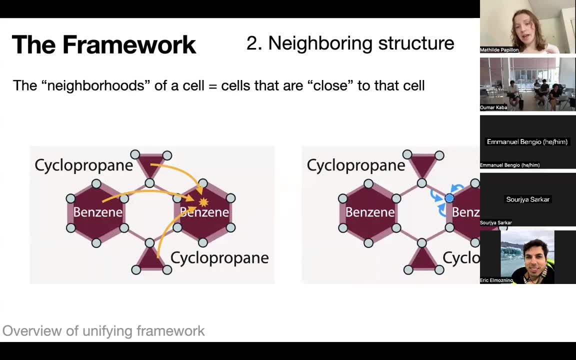 Okay, great. So coming back to neighboring structures, these are going to lay out- you can imagine, kind of the roads that our messages can take on our domain. So, for example, this benzene in this molecule might have the neighbors of all the other faces in the molecule, the two cyclopropanes. 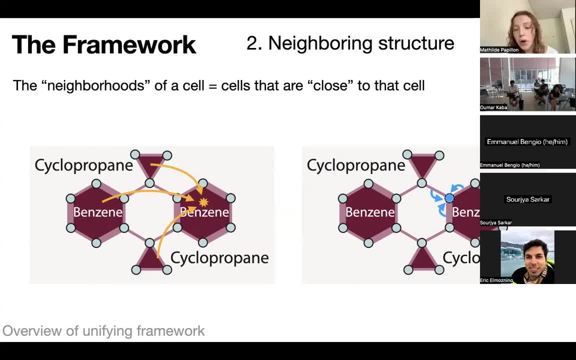 and the other benzene ring Or, for example, this node on the right-hand side could have neighbors of the edges that are connected to the node. My point here is that the choice of neighborhood is pretty arbitrary and will seriously affect how your topological neural 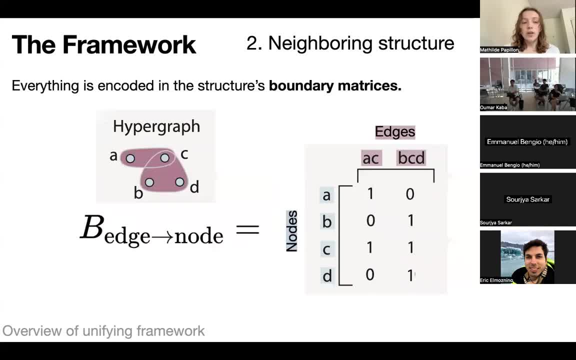 network, processes, information. So to encode these roads we use something called a boundary matrix. perhaps something that's called a boundary matrix. Maybe you've heard of this before with graphs. Another word for it is incidence matrix. In a boundary matrix you are encoding. 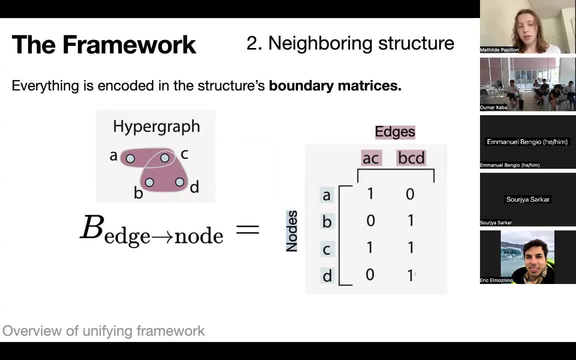 the nodes, or cells or whatever it is that you're looking at, in this case the nodes that are on the boundary of the edges. So here in this hypergraph, we have two edges, aC and bCd. which nodes bound, which edges? You can do the same thing with this combinatorial complex. 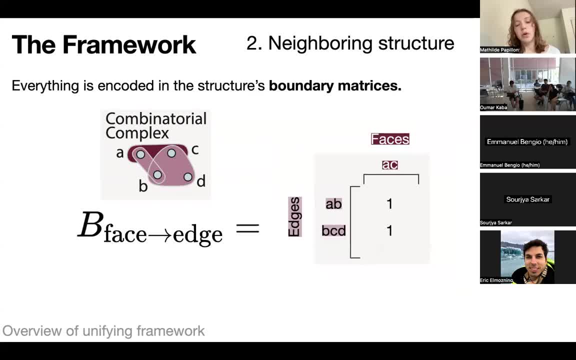 for example, and you can do it for higher rank. So here we're encoding which edges are on the boundary of the AC face in our combinatorial complex. You can think of the boundary matrix as kind of a Lego building block that we will use to build up our neighboring structure. 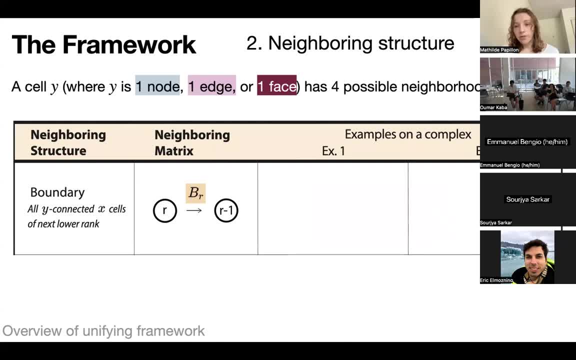 Specifically, there are four very common types of neighborhood structures that people use in the literature, And we'll go through all four and see examples of what they look like on a domain. So the first is the boundary neighborhood structure, which, somewhat obviously, is simply the boundary matrix that I showed you before, where we are looking at. 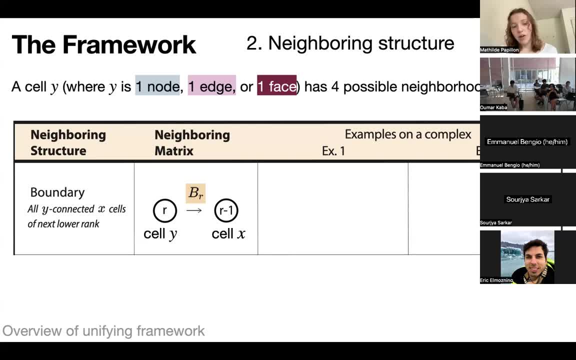 the cells of lower rank that are on the boundary of our initial cell. So, for example, the boundary of this edge y are these two nodes, x, and the boundary of this face are these edges. And then we have our co-boundary. So in our co-boundary we're taking the transpose of 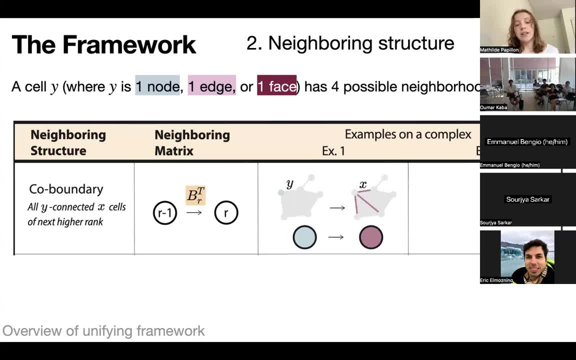 our boundary matrix And at this point we're looking at all of the edges that have y in their boundary, if that makes sense. So we're going up a rank instead of going down a rank. Another example is this face. So this face's co-boundary- sorry, this edge's co-boundary- is: 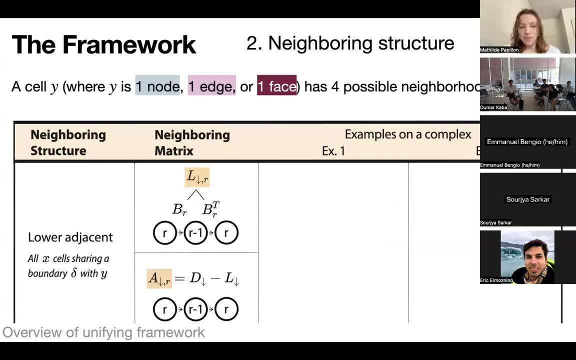 this face. Okay, Now, the next neighboring structure is called our lower adjacent structure, And this is all the cells that share a boundary with, So, for example, all of the edges that share a node that is also on the boundary of y. 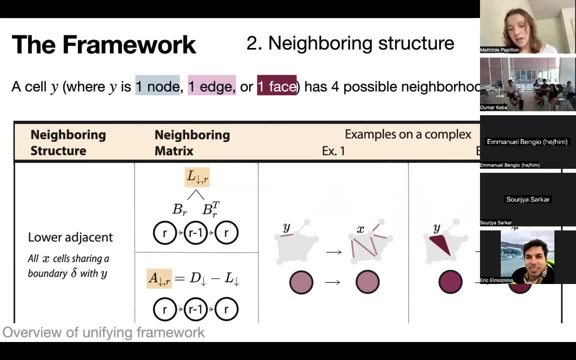 here. both of these faces share a boundary, share an edge with our initial phase y. And then the upper adjacent structure is similar, except now, instead of going through the boundary, we're going through the co-boundary. Okay, boundary, So we're going to go up a rank. These nodes share a co-boundary, ie are on the boundary. 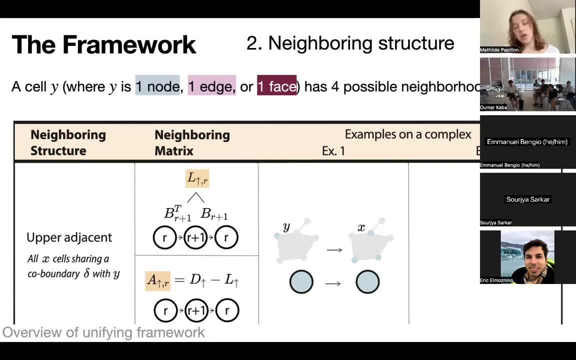 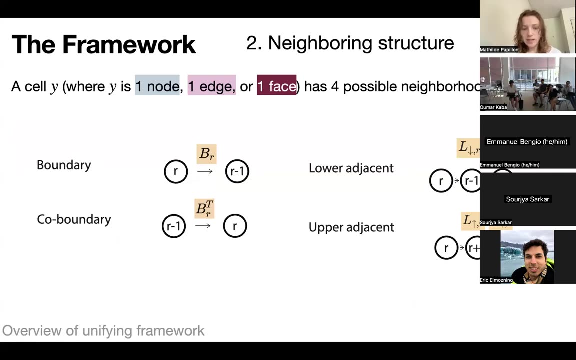 of an edge that y is also on the boundary of. And then these edges are on the upper adjacent neighborhood structure of this edge, y, because they share a co-boundary, they share a face with y. So these are four neighborhood structures and that might have been a little bit dense. 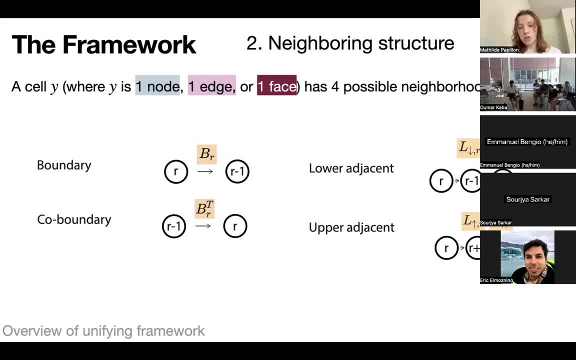 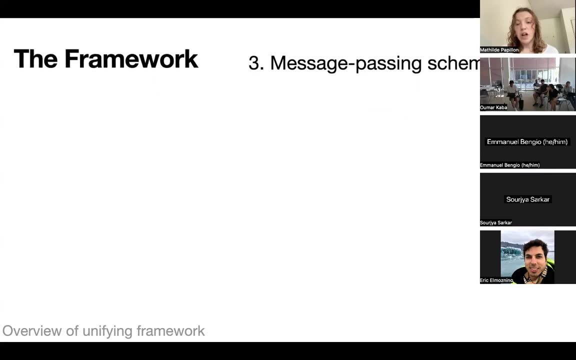 but basically all four neighborhood structures are just sets of roads that map possible ways for information to travel on your domain. Now we're going to use these neighborhood structures to build up our message passing scheme, which will specify exactly what information we're passing on our domain. So we're going to use these neighborhood structures to build up our 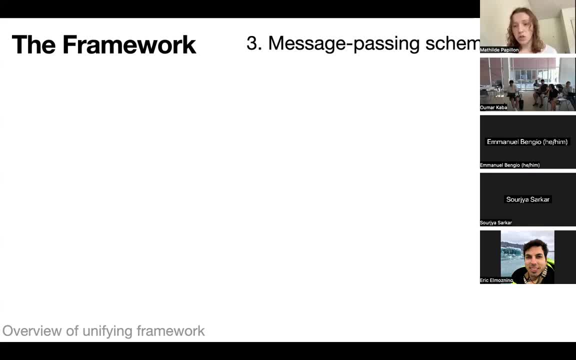 message passing and how that information is manipulated as it travels along the neighborhood structures. Okay, So to make this really simple, let's pretend that our initial layer t, we're going to represent all of the features on the nodes as this dot and we're going to represent 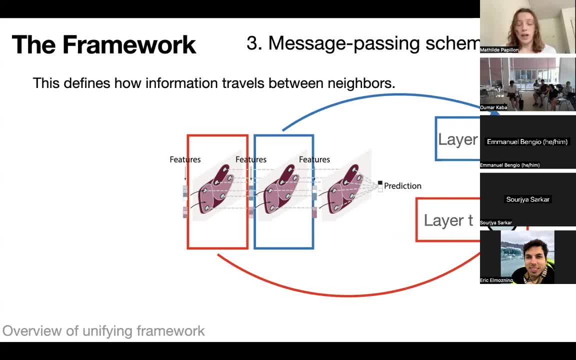 all of the information on the nodes as this dot for the next layer, and we're going to represent the operation of the node as this dot. So we're going to represent all of the information on the hands of the humans, the type in which humans bitten, the disposition and nature of these humans that will end up in this đang the network, So they can't. instead, we're going to have constant per300 0000 0000, 0000, 00000 m9 m6 when they find themselves in the H? t side of Yang Yi, but we're going to give them. the data, like the environment of the H, t side of Yang Yi. but we're going to want our message to even to remove that variation that sends message from layer t to layer t plus one and the other. اللهi, Mrs don't know that That only comes at one point. so 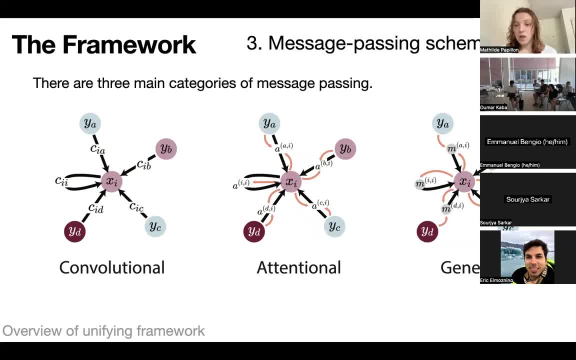 I'll send my second figure and the next one I'll send to my や t plus one as just an arrow between those two dots. Okay, so there are three main categories of message passing, and this is exactly the same as for graph neural networks. So maybe 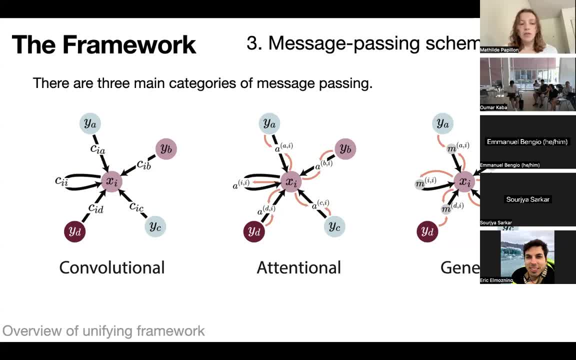 you're even familiar with this figure. In the convolutional case we are sending just linear multiplied versions of information on sending cells to our receiving cell. So c is some scalar that multiplies the feature on y and sends that to x. Information is aggregated through summation. It's basically just a matrix multiplication. 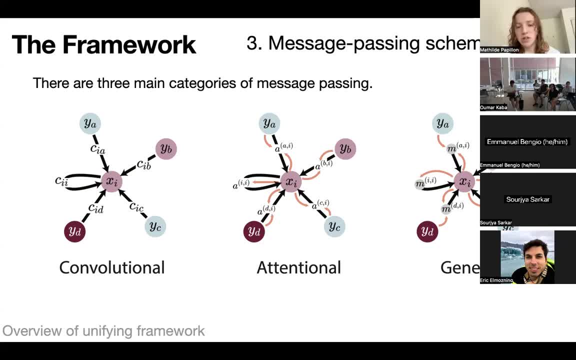 In the attentional case we will weight information by some weight learned, attentional weight a, And in the general case it doesn't even have to be some linear multiplication. so the possibilities are endless and we can also have attention in the general case. 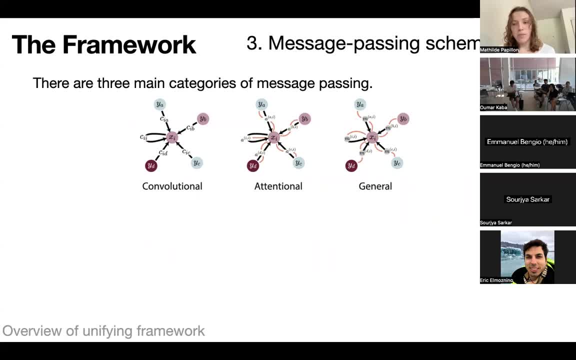 All right. so let's represent this with our little diagram that I showed earlier. So in the convolutional case, if we're sending a message convolutionally, we'll just have a black arrow, and that's how we'll represent a convolutional message. In the attentional case, we'll represent 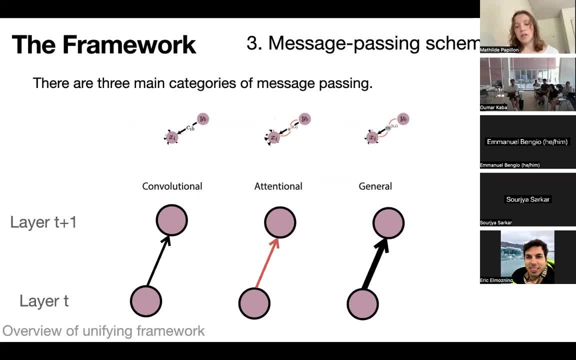 it as a red arrow and in the general case, we'll represent it as a fat arrow, And remember that the general case can also be attentional. Great Now, how do we actually send the message? through which roads? Well, that's our neighborhood. 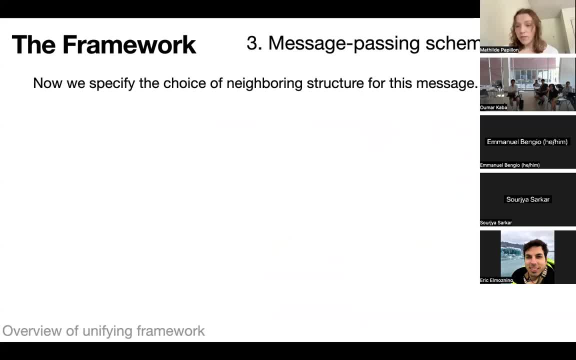 structure right. So we're going to specify our choice of neighborhood structure. Say, we're sending information from nodes to nodes, Let's look back at our four possible options. In this case, there's only one thing we can do, and it's the upper adjacent neighborhood structure. 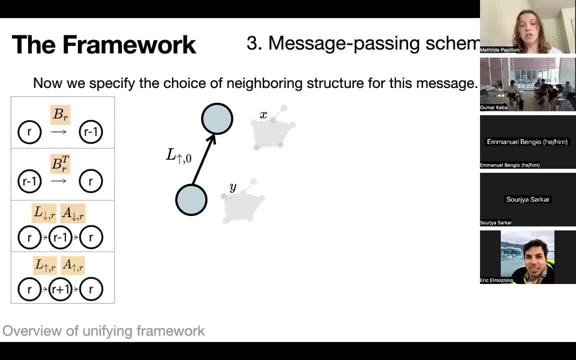 So in the upper adjacent neighborhood structure we will send information to all the nodes that share a co- boundary with our sending node Y. I would point out that this Laplacian is what you see in graph neural networks, if that means anything to you. 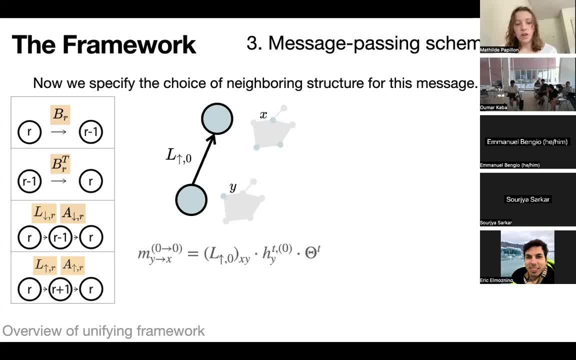 So L? up is just the regular Laplacian from graphs. Computationally, what this looks like is our weight matrix theta, which multiplies our initial feature on cell y, h, which multiplies our upper adjacent neighborhood matrix L up, 0 at indices x, y. Let's look at another example. If we have edges, 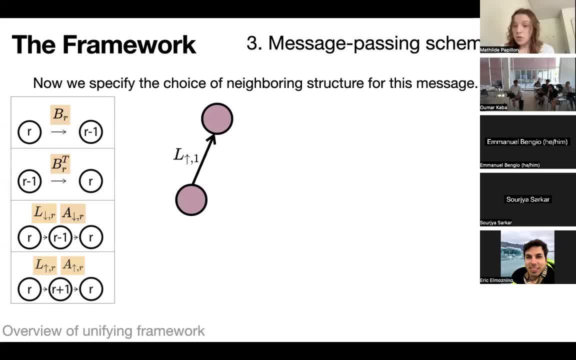 sending information to edges. well, we could still use the upper adjacent neighborhood structure. In this situation, we'll be sending information through faces and the message passing equation looks very similar. But we can also send information through the lower adjacent neighborhood structure. In this situation, we'll be sending information through nodes that are on the same. 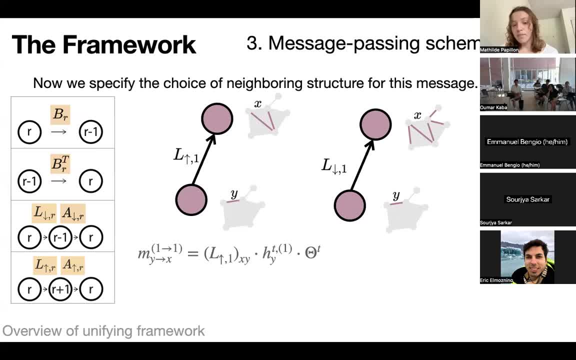 boundary as y. Message passing equation still looks very similar, but notice now that we're sending information through nodes that are on the same boundary as y. We're sending information inherently to different parts of our domain. Okay, what if we're switching ranks? What if we're sending information from a node rank 0, to an edge rank 1? There's only. 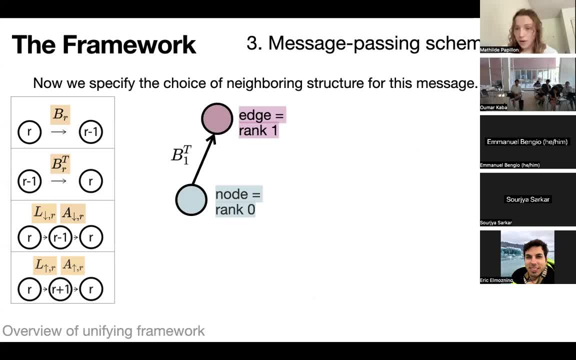 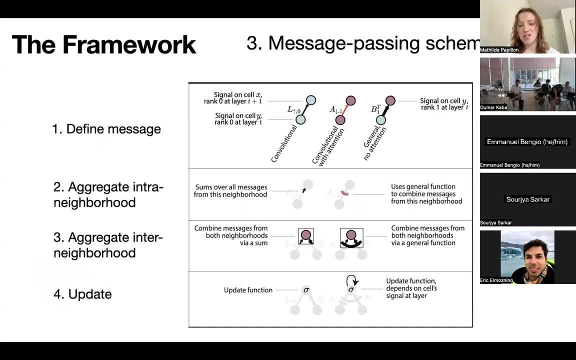 one neighborhood structure that can do this, and it is the co-boundary. So in this situation, we're sending information from a node to an edge, and this is what the message passing equation looks like, And that gives you an idea of the first step of message passing scheme. So the first step, 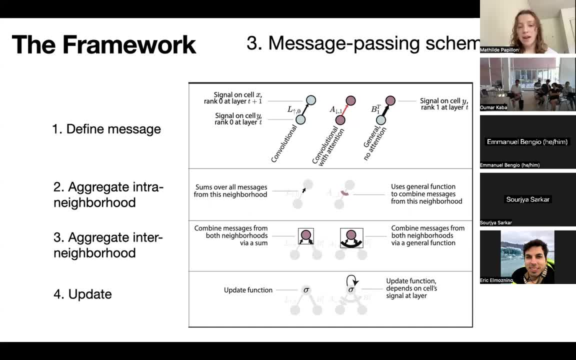 is to define the message, ie, pick your type of message and pick your neighborhood structure. The second thing we have to do is aggregate information over our neighborhood. So what if I have multiple cells in a boundary that are all sending information to one cell? Well, I can either. 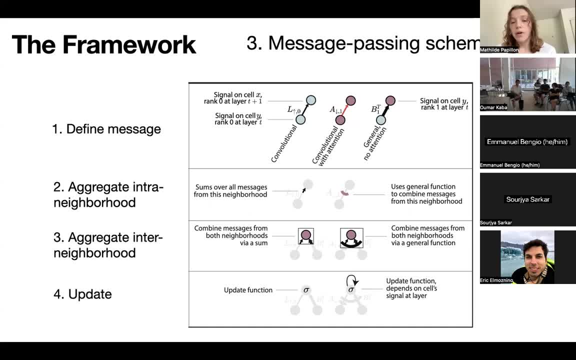 add all of these messages with just a simple arrow, or I can do something more complicated. I can take an average, I can take a weighted sum. In that case, we'll put a little banana to indicate that some aggregation more complex than a sum happened. Okay, now we have to aggregate information. 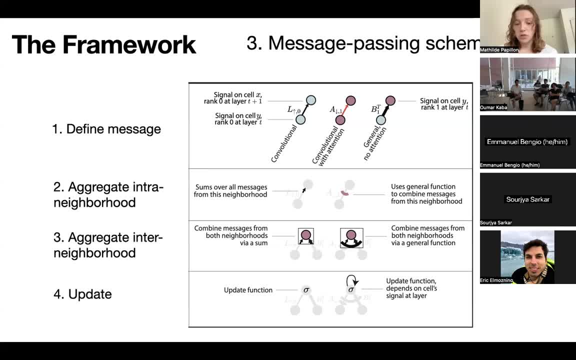 across multiple neighborhoods. What if, in your topological neural network, you're sending information through nodes that are on the same boundary as y? What if, in your topological neural network, you're sending information through nodes that are all sending information to one cell? 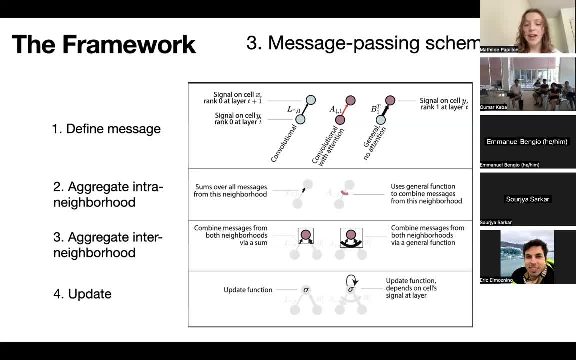 What if, in your topological neural network, you're sending information both through a co-boundary and an upper adjacent neighborhood structure to the same cell? Well, you have to figure out how to aggregate those messages. So again, we can just decide to sum these messages, in which case we'll 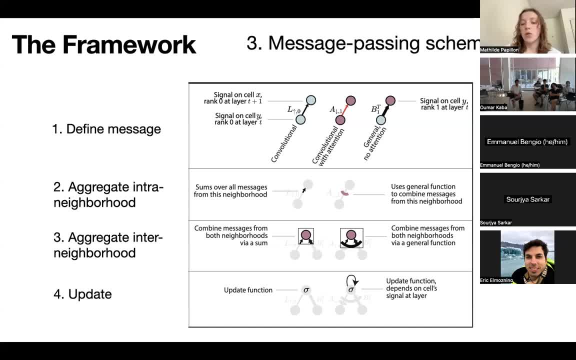 leave our arrows blank, or we can decide to do something more complicated, in which case we'll put another banana, And the last step is the update. The update function can be something as simple as a sigmoid, for example, that you send your last message through, or it can be something a little. 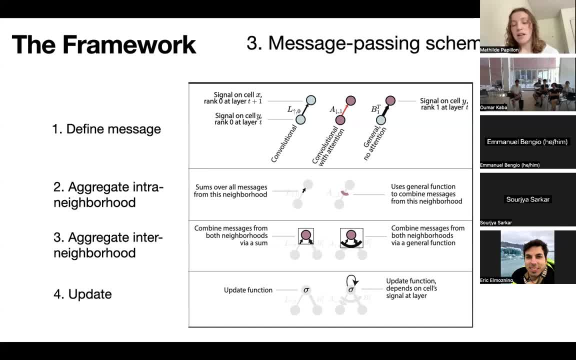 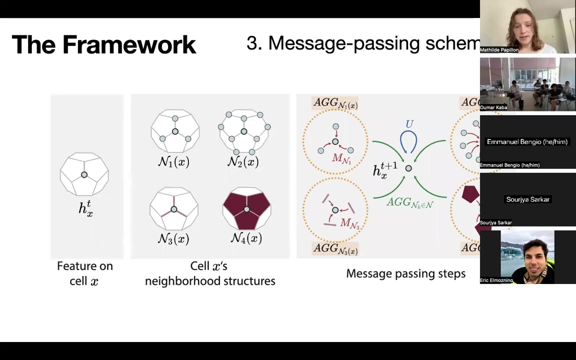 bit more complicated. that depends on the feature, initially on your receiving cell. So maybe you have some other weight matrix that will multiply your initial cell feature and add that to your new feature that you've aggregated from all of the neighborhood structures. This is a little bit dense so I made this figure to visualize the four steps of the message passing. 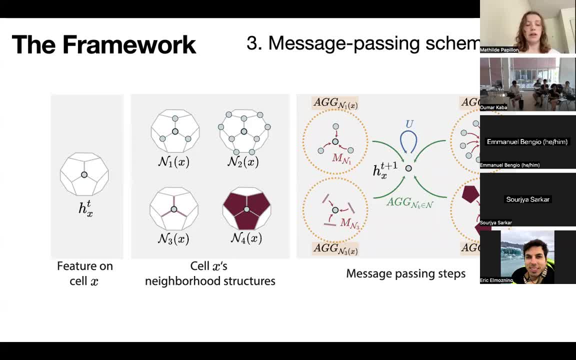 scheme. So say, we have some initial cell x, this node x, and we pick four neighborhood structures. So in this case the first neighborhood structure is those three nodes, the second is all of those nodes, the third is the three edges and the fourth is the three faces. So we're going to 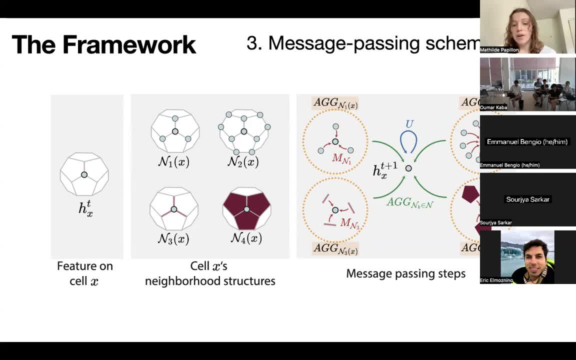 do the same thing over and over again. So we've got our neighborhood structures. The first step is going to be in red, where we send information from each neighboring cell to our receiving cell. The second step is going to be aggregating over the neighborhood, So, for example, summing: 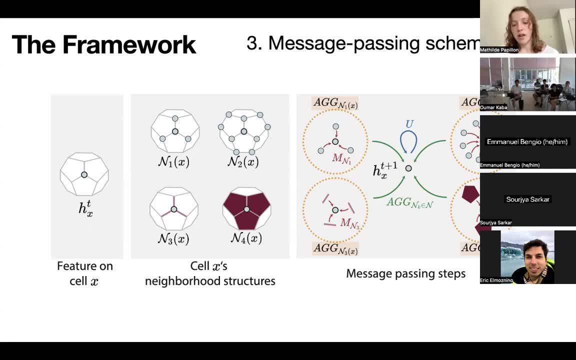 information over all three nodes in the first neighborhood or all three faces in the fourth neighborhood, And then the third step is going to be aggregating information from all four neighborhoods by some aggregation function in green, And then the last step will be an update. 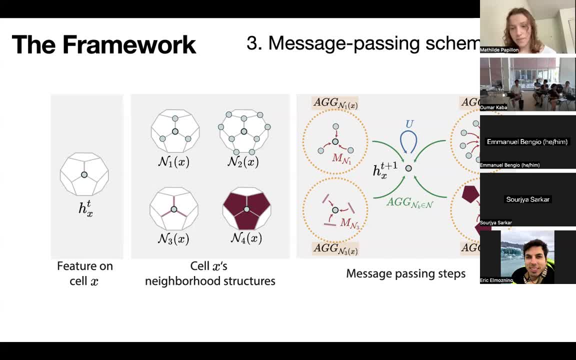 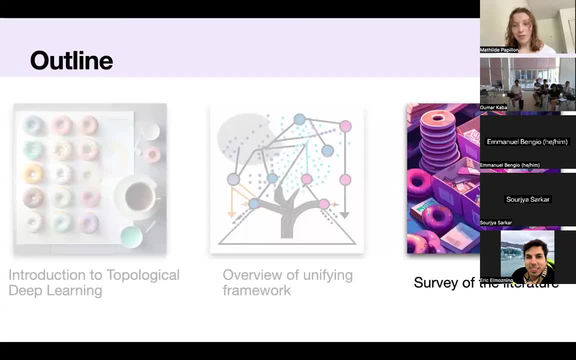 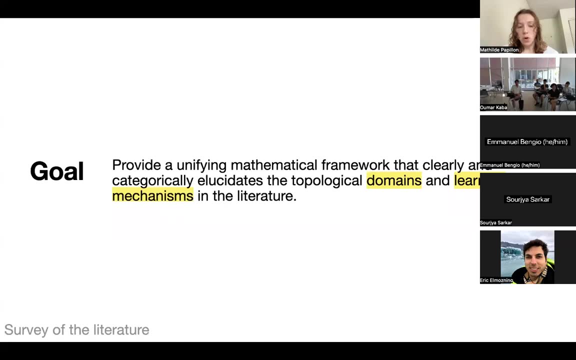 that occurs on the receiving cell, And again, the update can be something as simple as a sigmoid. Okay, so we've got our framework and now we can apply it to look at the literature. So this was our original goal was to elucidate the topological domains and learning mechanisms. 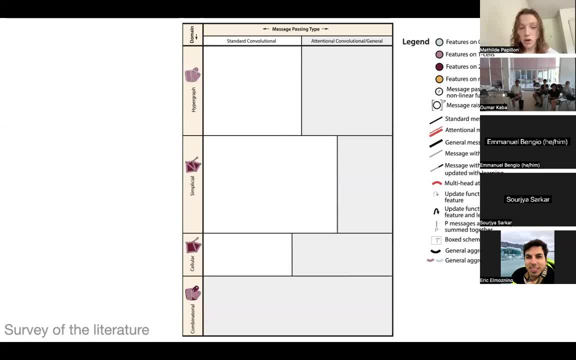 in the literature. So, to use our framework, let's divide up the literature into categories. Domains are the rows and learning mechanisms are the columns where you can either have a convolutional message or a tensional or general message in gray. Let's start with the hypergraph domain. So the hypergraph. 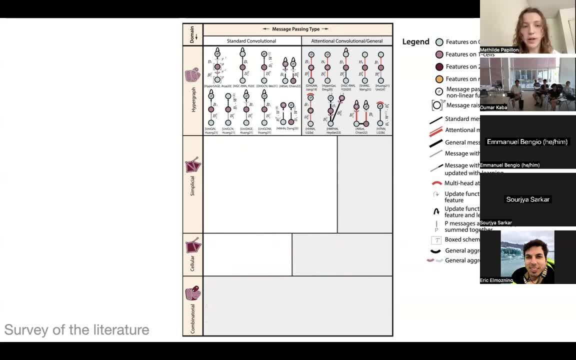 domain is the oldest domain in topological literature And it's the oldest domain in topological deep learning And the first so for a while. what people did was collapse hypergraphs into graphs and then send the graphs through graph neural networks. But in that collapsing process, 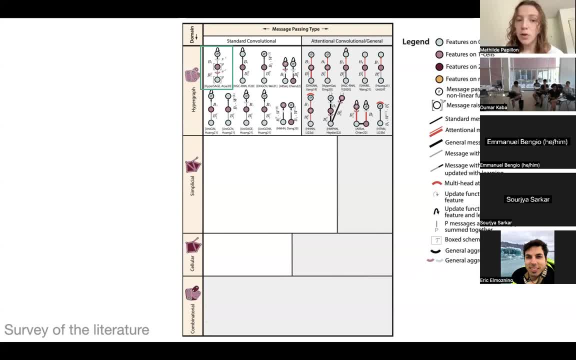 they would lose a lot of important structural information about the hypergraph. So the first paper to preserve hypergraph structure and send it through topological neural network came out in 2020.. people in the hypergraph community have done a really good job at generalizing graph results. 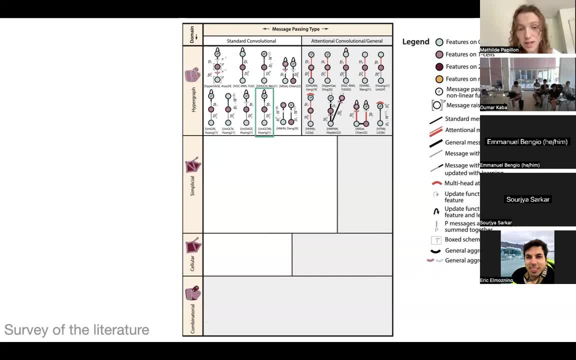 to hypergraphs. So an example of this is UniGCN2, which generalizes GCN2,, which is a graph neural network, to hypergraphs. And this is a really special neural network because it addresses the over-squashing problem, which is a big problem for graphs, just as it is for topological neural. 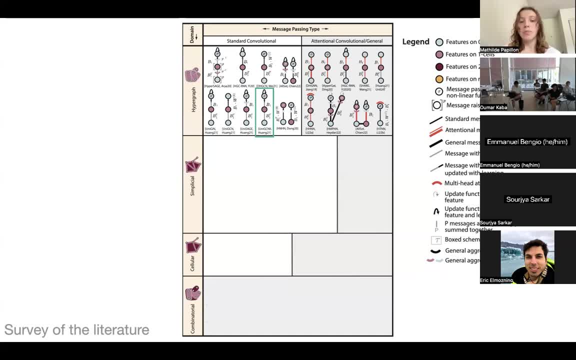 networks And they showed that they could apply the same mechanisms in GCN2 to address over-squashing in hypergraphs. Allset generalized hypergraphs to transformers, which is another example of generalizing important results from traditional discrete domains to topological domains. 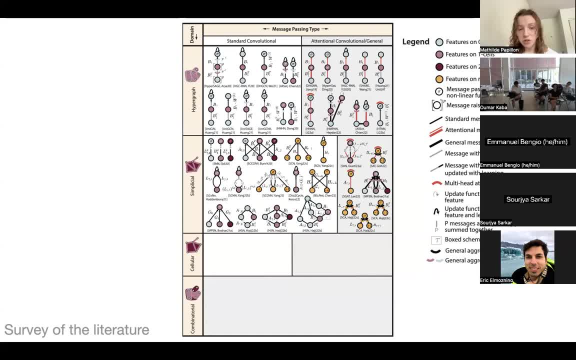 And then the next domain that we get is the simplicial complex domain. The simplicial complex domain has strong roots in the signal processing community, So people in signal processing were thinking about simplicial complexes a long time ago And the first neural network that was trained. 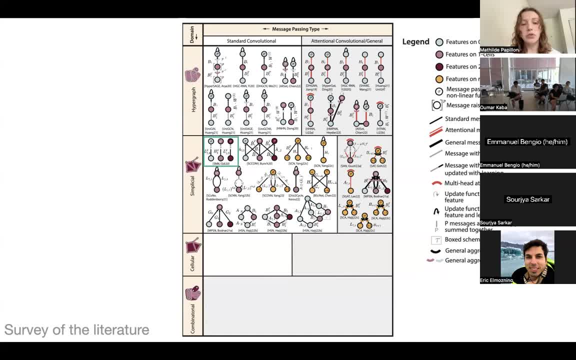 on this domain came out in 2020.. And you'll notice that in this neural network it looks a lot like a graph neural network, in the sense that it's not a graph neural network. It's a graph neural network where nodes only send information to nodes, edges only send information to edges and faces only. 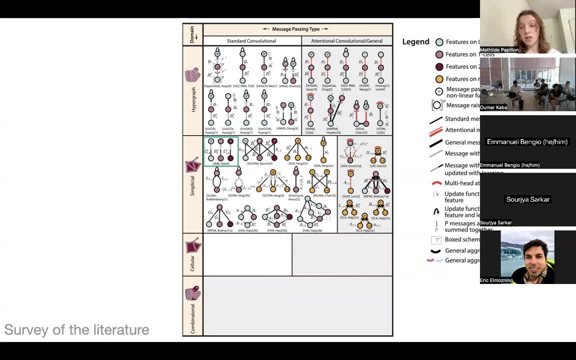 send information to faces through mostly just Laplacian neighborhoods, which is characteristic of a graph. neural network Bunch came out with this neural network not long after which, unlike the first neural network, is now sending information across different ranks, which turns 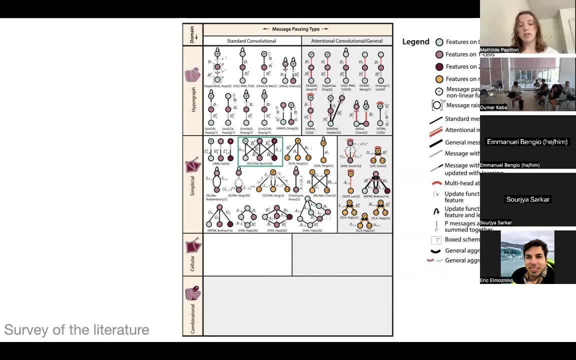 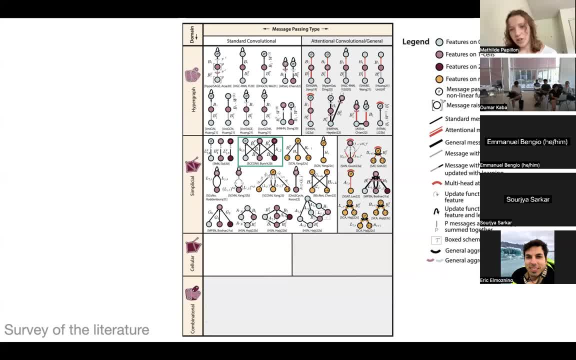 information from nodes, edges and faces, et cetera. And then I'd like to point out high skip networks, which came out in 2022.. High skip networks were the first network to have this sort of double neighborhood structure in one layer that is similar to the hypergraphs. 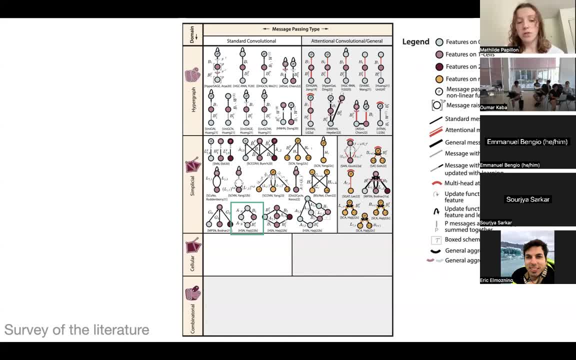 So in this situation, in one layer of our topological neural network, we're sending information through a first set of neighborhood structures, So the node sends information to both nodes and edges, and then through a second set of neighborhood structures. So again, 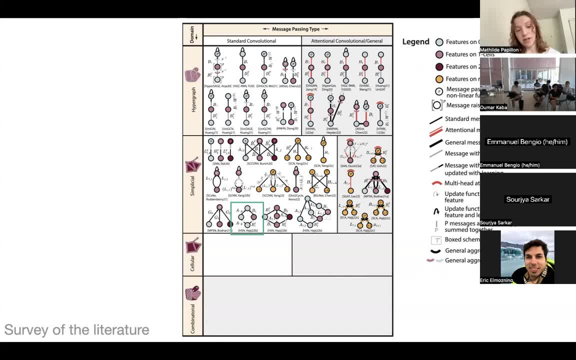 the upper adjacent neighborhood structure and then the boundary, to take information back from edges to nodes And, as you can see, things get infinitely more intricate as you go along. You add neighborhood structures to your layer. I'd also like to point out attention in simplicial. 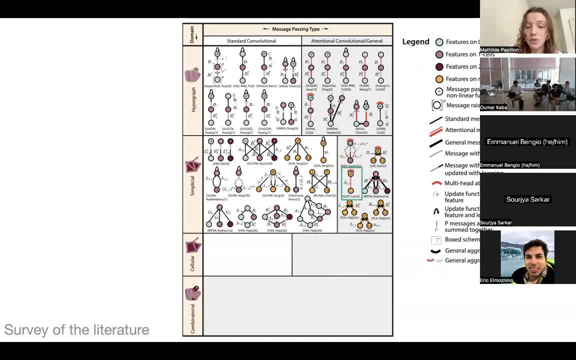 complex neural networks. This neural network, specifically SGAT, is the only topological neural network as of yet to be heterogeneous in the sense that it is capable of dealing with features of different dimensions, And it's quite interesting That this has not been done more so far. Okay, In the cellular case, we have less. 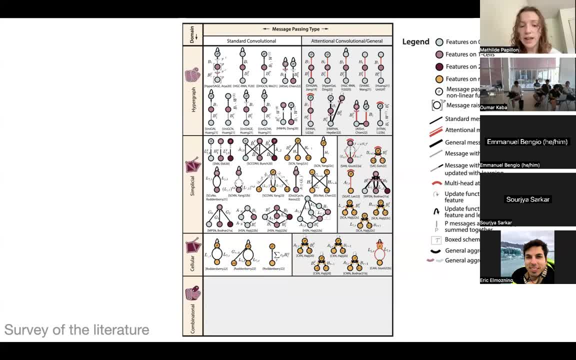 much less neural networks than in the simplicial and the hypergraph case And you'll notice a lot of strong parallels with the simplicial case. So, for example, this neural network with the two Laplacians on either side looks a lot like the. 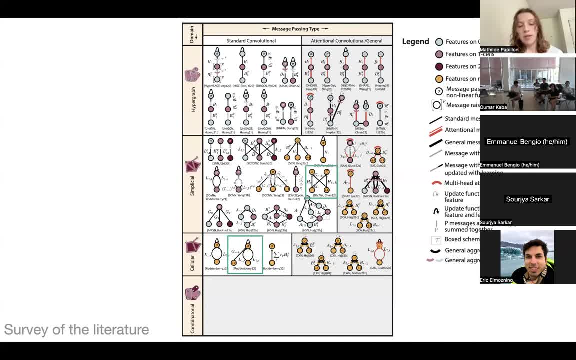 simplicial network, Scone. This neural network has the same idea as BSCNNet, where you're sending information from some rank K to any rank R through this pseudo neighborhood structure. And finally, I'd like to point out the only attentional neural network in the cellular. 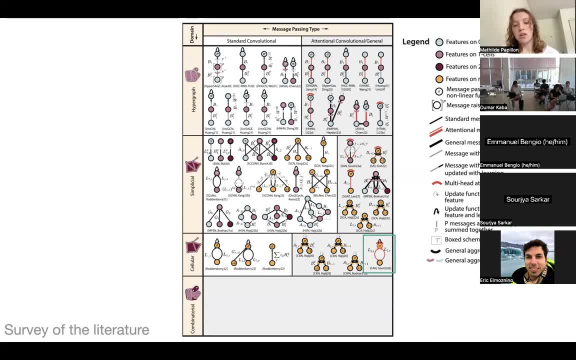 domain so far again looks a lot like the top left attentional neural network in the simplicial case. And finally, our last domain is the combinatorial domain. There's one paper that has implemented this domain so far, so a lot of work remains to be done in terms of understanding the advantages. 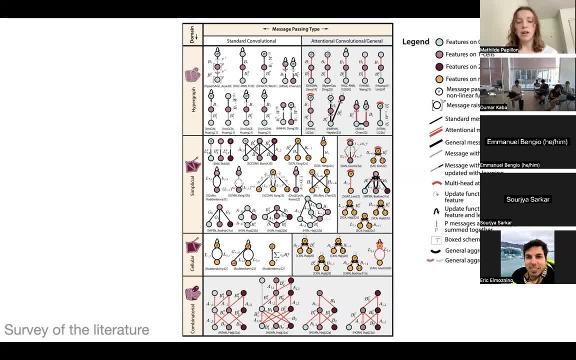 of this theoretically much more expressive domain over cellular and simplicial and hypergraph domains And that's kind of an open question for the field to answer in the coming years. I hope Broad comments on performance is that everyone agrees. So the hypergraphs, the simplicial, 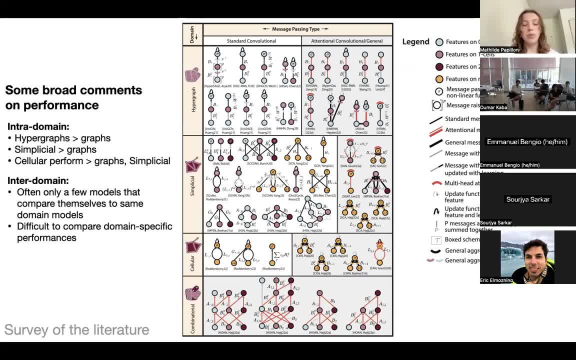 and the cellular networks all perform better than graphs at the tasks that they are trained on. So things like Like semi-supervised node classification, link prediction, graph classification. However, you'll notice that there's very little inter-domain comparison. So, for example, 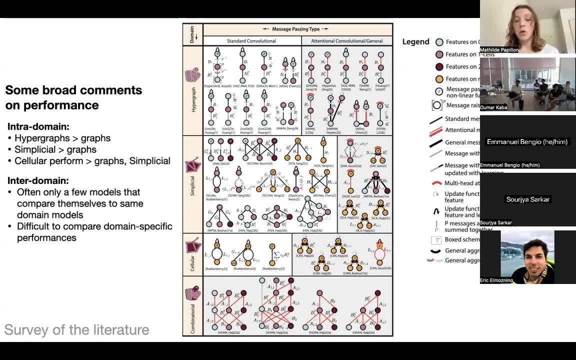 within the hypergraphs. it is very difficult to know which hypergraph model performs better than another hypergraph model at the same task, because the field is still very focused on benchmarking. The purpose of this is to kind of to evaluate whether or not sure-ness is actually really. 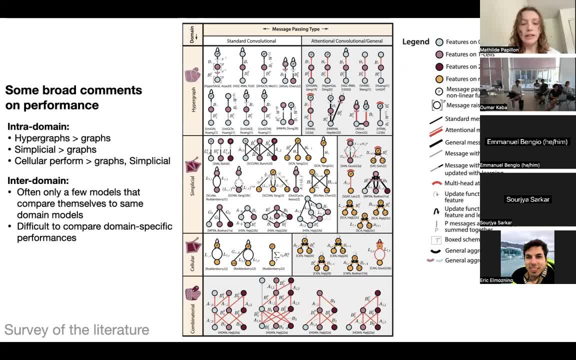 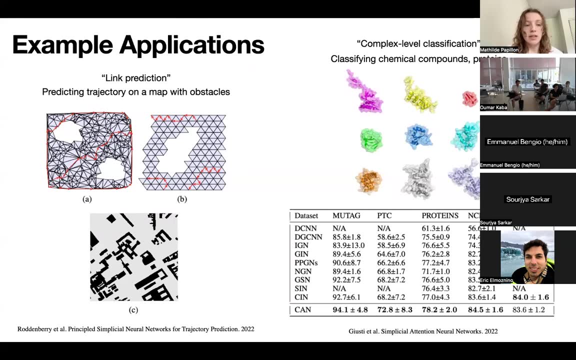 different for the query itself compared to graph neural networks. We hope to kind of address this with the literature review and hopefully give people some hints as to which models might be better suited to their task than another topological model in that same domain. So some example applications of what people have done. 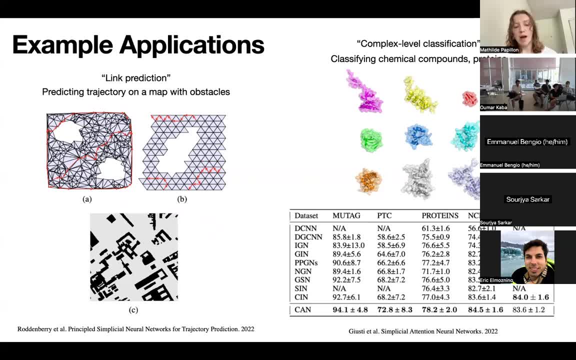 map C: at the bottom there is a map of Berlin where the dark spots represent obstacles in the city, and it turns out that a simplicial, complex neural network is very powerful for encoding the topological structure of such a map and predicting trajectories that take into account. 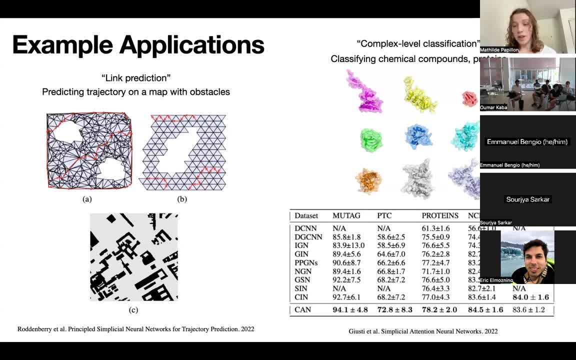 the obstacles that are encoded as topological features of a map. Another example of an application is classification of chemical compounds and proteins. You'll see here that this simplicial, complex attentional neural network does really well, much better than state-of-the-art. 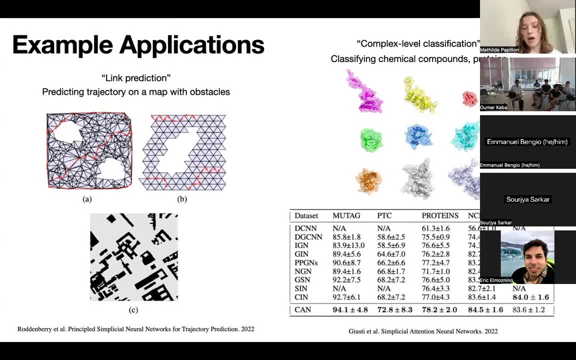 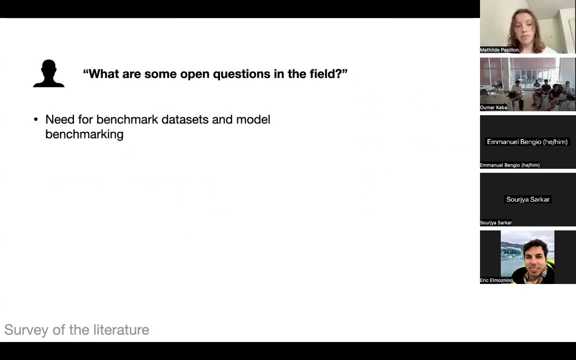 graph neural networks, at classifying at a series of proteins and nitrate compounds, I believe. all kinds of things. Okay, so what are some open questions? Like I was saying earlier, we need better benchmarking. we need better data sets that are suited to topological neural networks and are not just 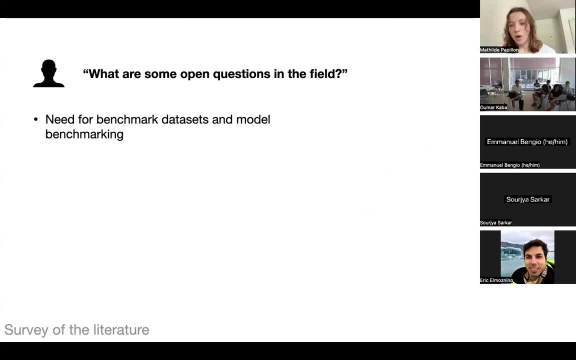 lifted graphs that people are sort of arbitrarily choosing how to lift, and then we need better addressing of the over-squashing problem. This is an active area of research in graph neural networks and in topological neural networks. so far we've only seen two approaches at solving the problem. 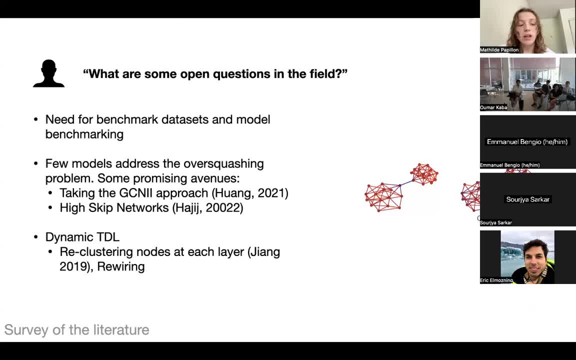 And finally, dynamic topological deep learning has been mostly done in the hypergraph community, so there's no neural network in the simplicial, cellular or combinatorial cases. that changes the domain at every layer, And I would point out that dynamic graph neural networks are very common. 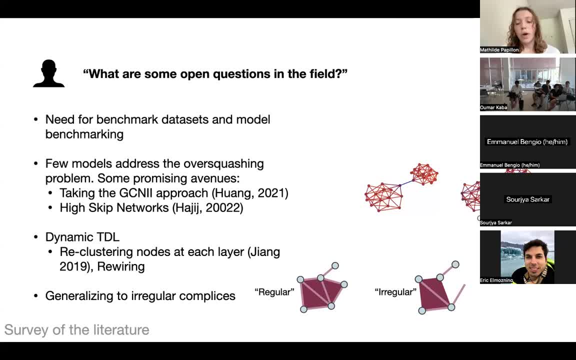 And lastly, while there's this idea of irregular domains, where, for example, you'll have a face that is not entirely bounded by edges but rather maybe just bounded by nodes, and right now, the computational methods that we use to send messages through neighborhood structures make such a domain kind of difficult to use- 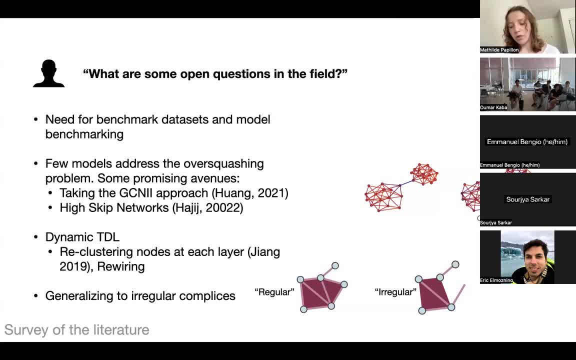 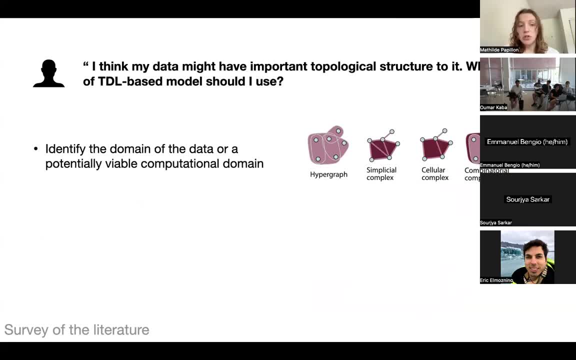 even though an irregular domain might be a much better representation of your data set. Okay, so what if you think your data has some topological structure to it and want to use a topological neural network? Well, the first thing you want to do is identify the domain. 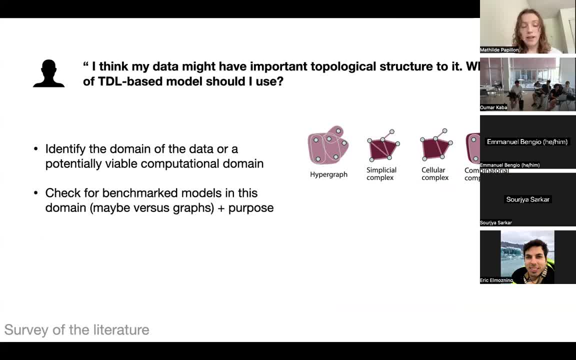 that you think is best for your data set. The second thing is looking at all the models that exist in the literature and then looking at all the models that exist in the literature and finding one that is benchmarked ideally versus other models in that domain. 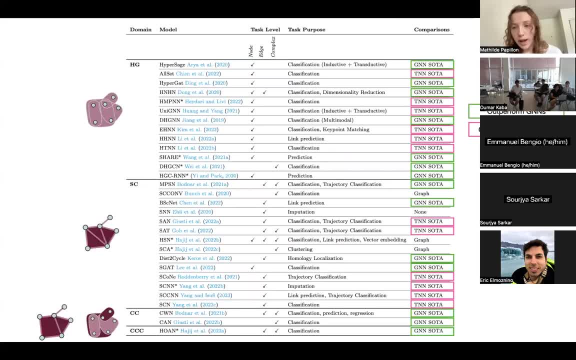 and also suits your purpose. So in the literature review we have this big table that tells you what every topological neural network has been trained to do, as well as its level of benchmarking. So in green are neural networks that do better at. 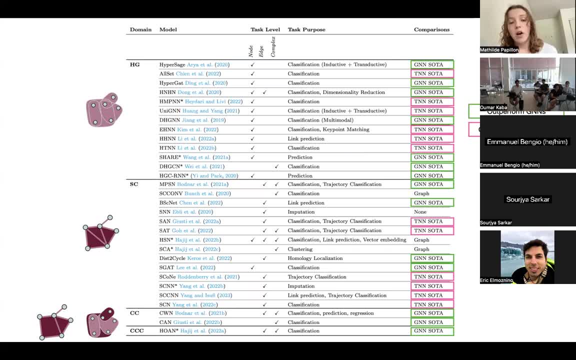 graph. neural networks state-of-the-art and in pink are neural networks that have been proven to do better than topological neural network state-of-the-art, which is a more powerful statement, And you can see all of the different tasks that people have trained their 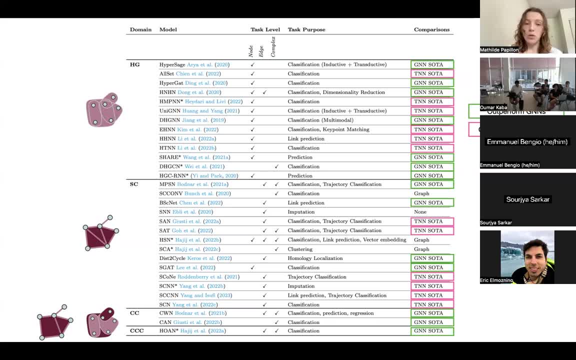 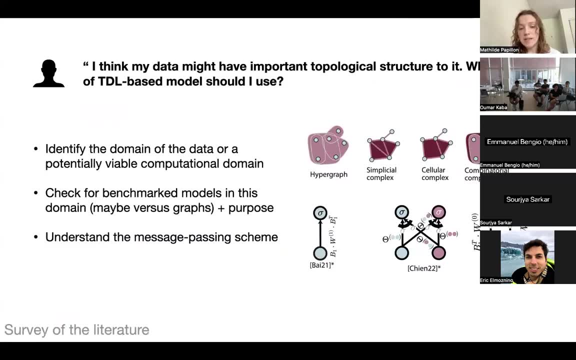 neural networks to do at the node level, the edge level and the complex level. The next thing is understanding the message passing scheme. There are, of course, the tensor diagrams that are used to do that. So the first thing you want to do is look at the message passing. 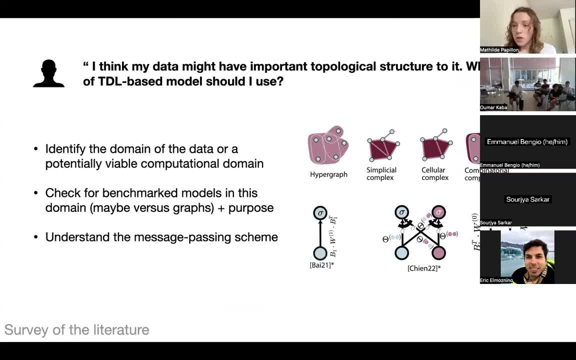 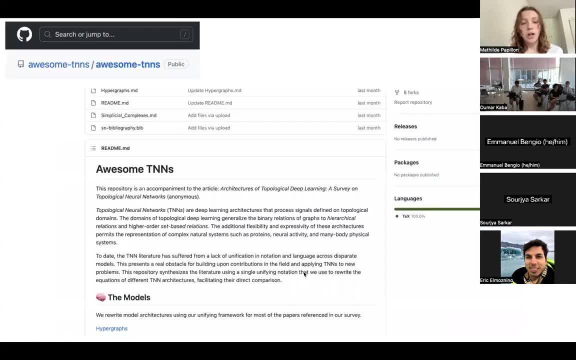 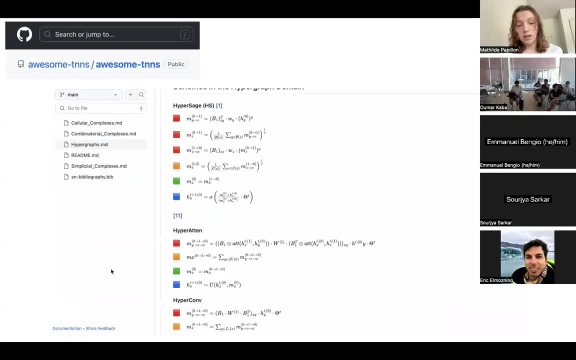 equations. So, for example, these are the programs that I showed you today that you can kind of see what's going on just visually. But you can also check out our repo, AwesomeTNNs, which encodes all of the message passing equations for all of the models in the literature review. So, for example, 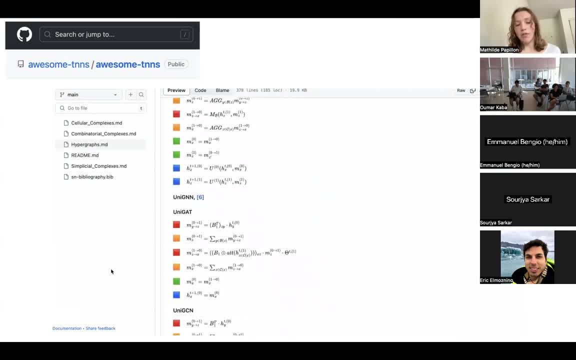 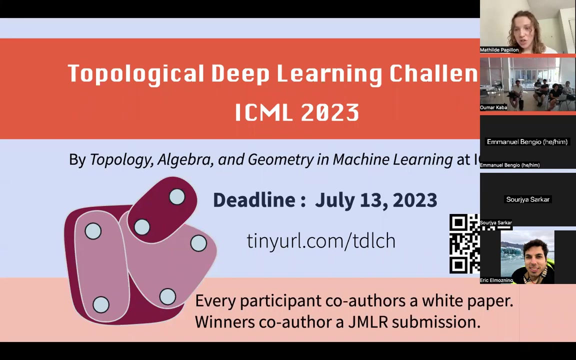 these are all of the message passing equations associated to each hypergraph neural network and they're all classified, they're all color coded by the color corresponding to the step in the message passing scheme. And the last thing I want to bring up is this challenge that we just announced last week: the topological deep learning challenge. 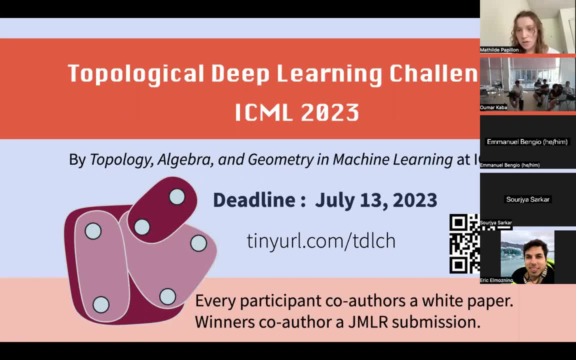 hosted at ICML. It is an awesome opportunity to get your hands on some topological neural networks. we are asking people to implement models that already exist in the literature, using Topo Model X, which is a package for building topological neural networks. 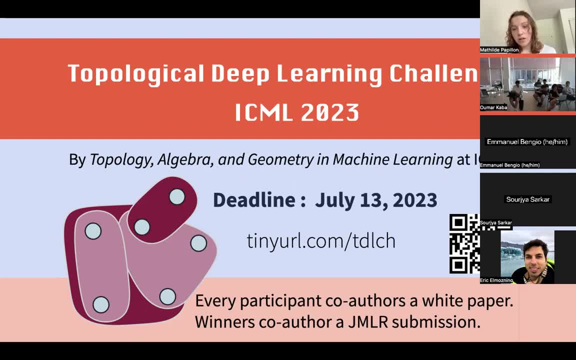 And this is really exciting because if you participate, you're guaranteed co-authorship on a white paper and winners get the chance to co-author a submission to the Journal of Machine Learning Research. You don't need to be registered to ICML, you don't need to. 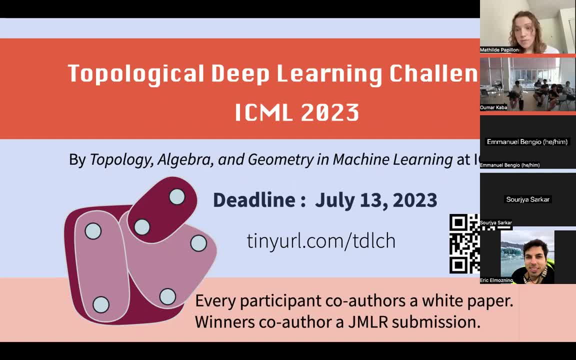 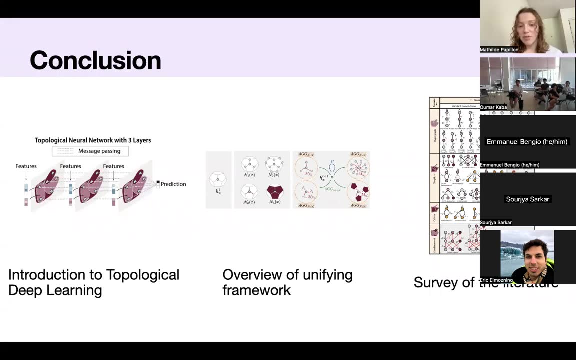 have any experience in the field. we accept teams and the deadline is July 13th, So I really encourage you to check it out if you're interested in learning more about the field. And to conclude, we looked at what topological deep learning was built up- a framework- and then 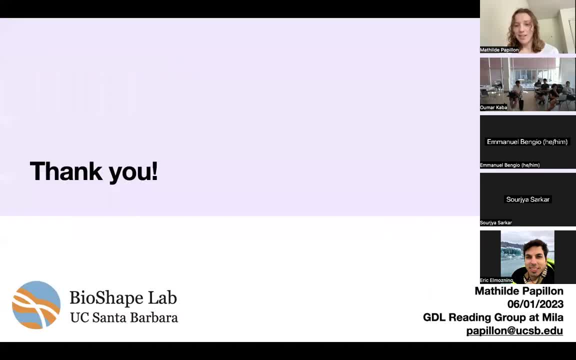 used that framework to break down the literature. Thank you, and I'm happy to take questions. So, thank you. this was really an amazing talk. We learned a lot and, yeah, I have questions. So, yeah, I'll start. So my first question would be: 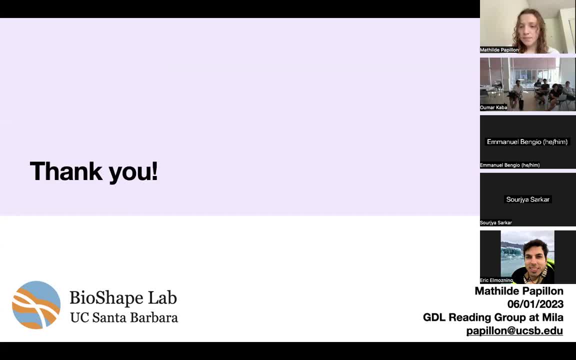 I saw that in your classification and in your survey you did not include. 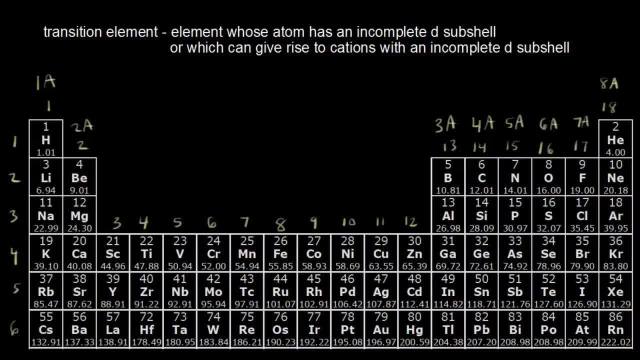 In the last video we saw the classification of elements into groups on the Peer Eye Table and we stopped with the definition for a transition medal. There are two ways to think about transition medals. One way to think about it would be when some teachers say transition medal. 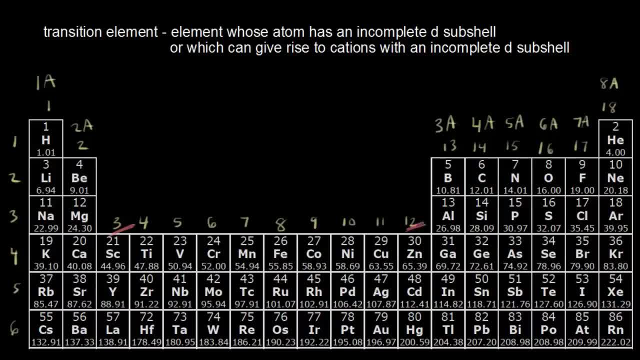 they're talking about elements found from Groups 3 through Group 12.. All of the elements in here. some people consider these to be the transition medals. These are the elements found in the D block. We're talking about D orbitals here. 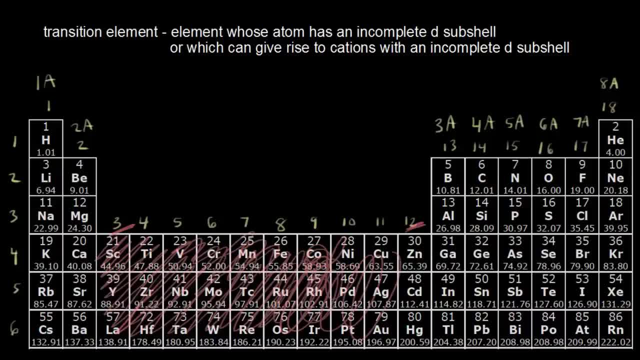 You have to understand electron configurations for this video. That's one way to think about the transition medals, but that way is maybe a little bit too general sometimes. There is another definition which you'll find on the IUPAC website. IUPAC is an acronym for International Union of Pure and Applied Chemistry. 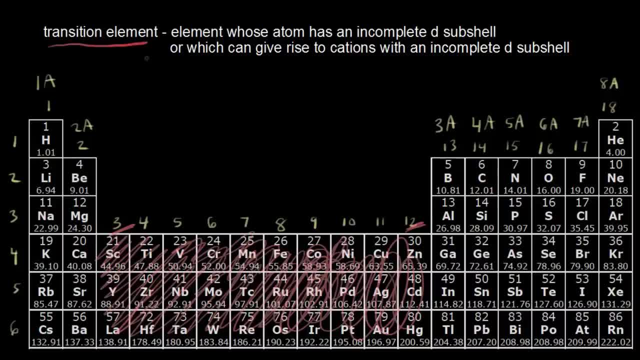 They say that a transition element refers to an element whose atom has an incomplete D subshell. When you're talking about the D orbitals, we already know there are five D orbitals and each orbital holds a maximum of two electrons. Five times two is ten.